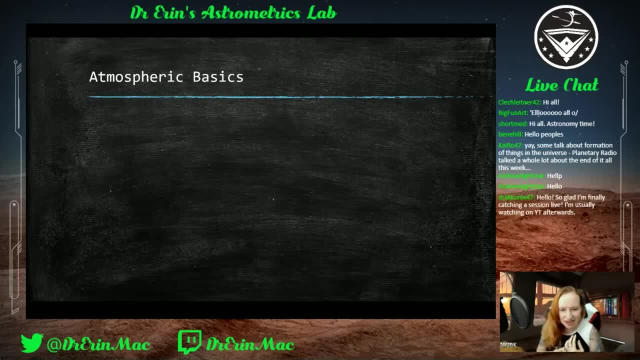 Earth right now. So yay, Dracorex, happy to have you, Yay. So some basics about the atmosphere, And the reason I remembered to hit record is because my parents watch this and my dad's an atmospheric scientist. So no pressure, They're not watching it now, but they watch it on YouTube. So 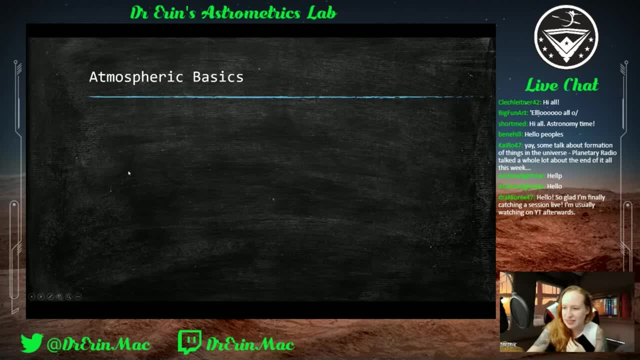 hi, mom and dad. All right, So some atmospheric basics. What is an atmosphere? Now, this is again one of those things that you ask people And it's like: do you know what an atmosphere is? And everyone's like duh Yeah. 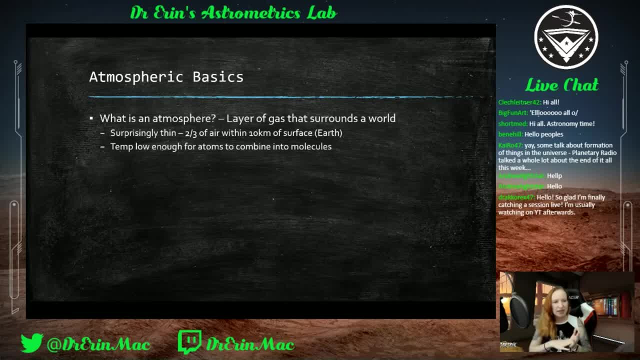 of course I do, But there's specific definitions to them And especially, I think this came up- I don't know if Andy's on, but Andy made this point in our Discord asking about the Moon's atmosphere, And is there actually one? So we'll mention that And it really comes from this. 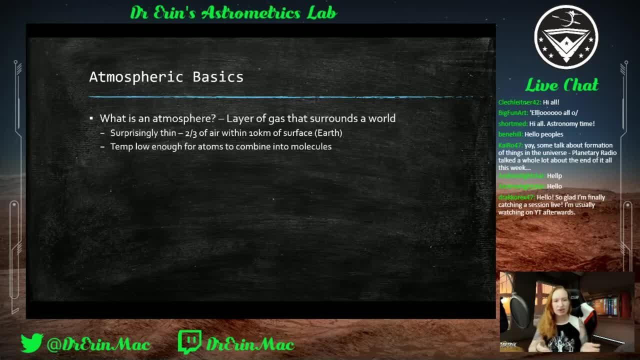 definition. What is an atmosphere? And it's just a layer of gas that's around the Moon And it's the world. It is shockingly thin, So two-thirds of the total air in our atmosphere on Earth are within just 10 kilometers of the surface. It just thins out a lot as you go up, And then the 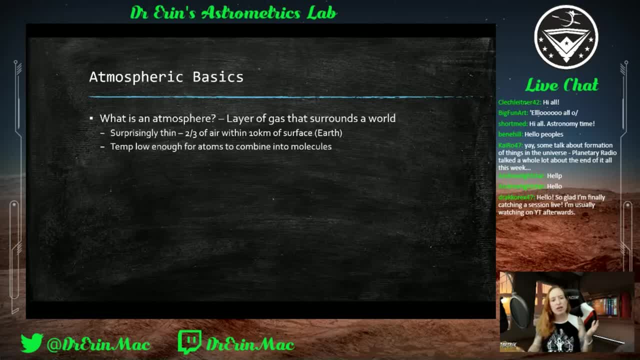 temperature typically, especially for Earth, is low enough that these atoms can combine to form into molecules. So that's why, if you hear about the fact that we have a nitrogen-rich atmosphere, but it's more N2 or O2 or CO2,. 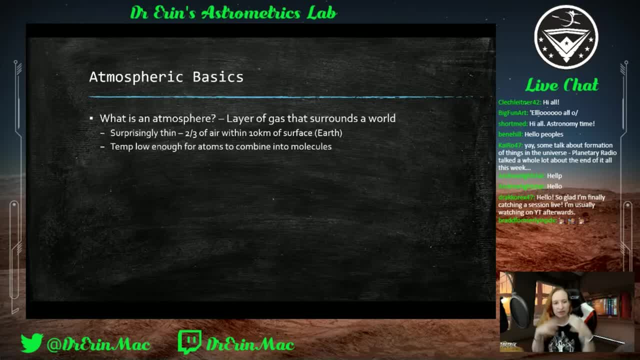 that's because the temperature of our planet is cold enough that those atoms can come together and form into molecules. To talk briefly about the thinness of the atmosphere, Hi Brad, I like your coffee sandwich there, Coffee and soda sandwich- A good analogy for how thin our atmosphere is compared to the size of the Earth. 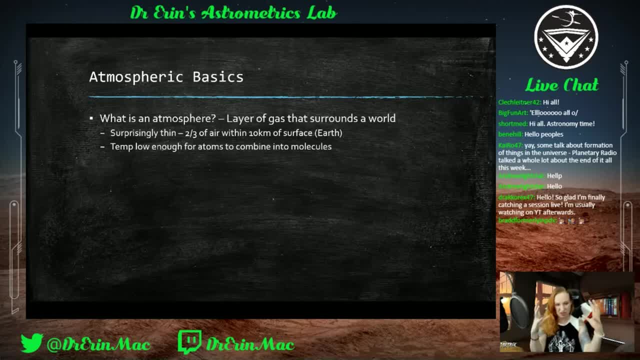 is if you can picture one of those just standard globes, you know. so about that big desk globes? That's how thin the atmosphere is relative to the size of the Earth. So a globe with just one note on top of it: That's the thickness of our atmosphere relative to the size. So 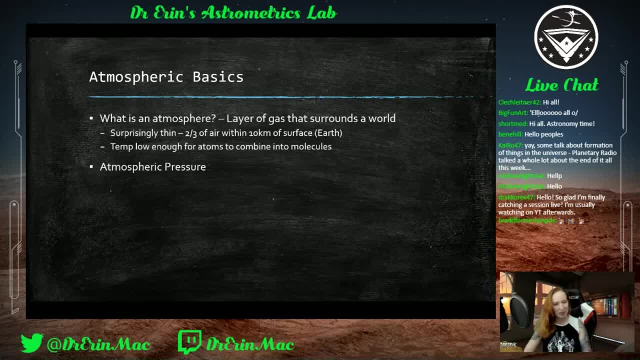 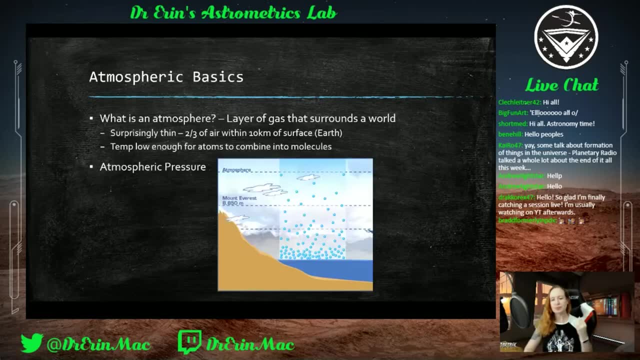 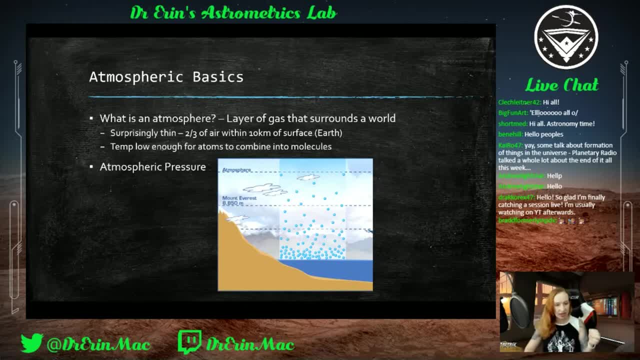 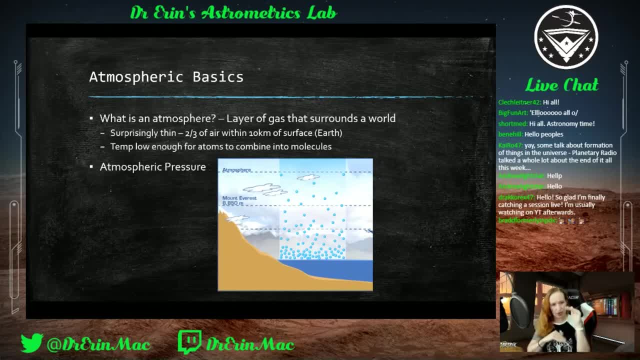 as you go higher in altitude. And so you know I said up front at the top of this chart that within 10 kilometres of the Earth's surface is two thirds of the air and it thins out really, really fast. Again. that's something that we kind of understand, but just trying. 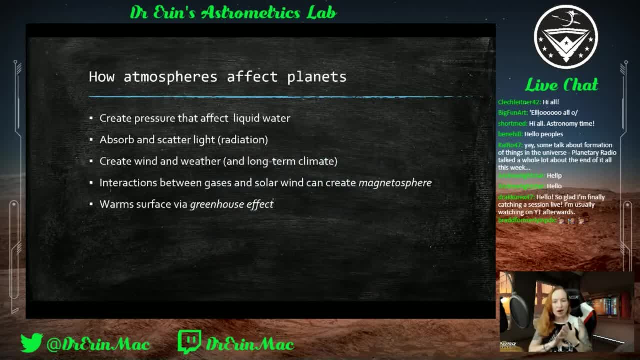 to wrap our head around how significant that actually is. atmospheres affect planets and why they're important. Lots of factors here. They create pressure that affects the liquid water. as I mentioned, They also absorb and scatter the light. So it's not just the fact that you know the atmosphere makes our sky blue, but the fact that 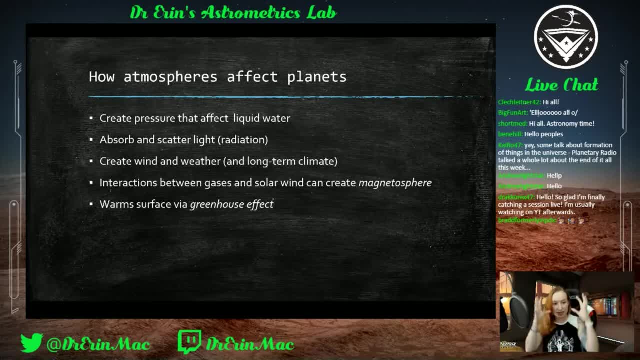 it protects us from radiations because it absorbs and scatters. Remember when we talked about telescopes And I'll show an image- I think on the next chart- about how far the different radiation gets into our atmosphere. that dictates where telescopes need to be. So if telescopes 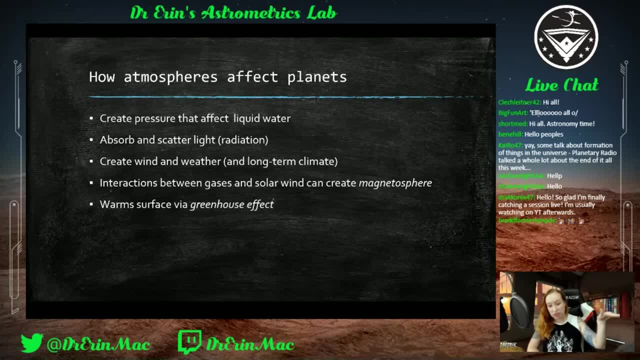 you know are more in the x-ray. they need to be outside of our atmosphere because our atmosphere absorbs x-ray radiation, which for us is a good thing. They create wind and weather and long-term climate of the planet, but particularly where we're in the middle of the world. So they're 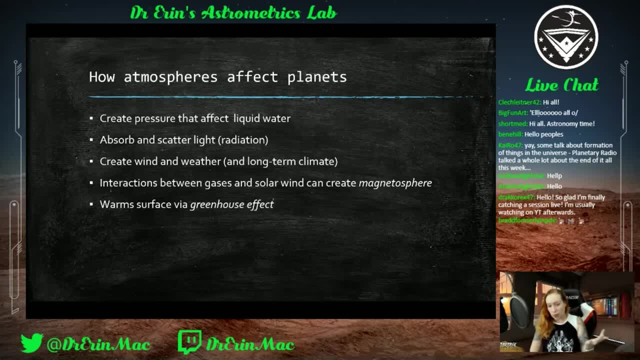 the surface of the planets Last week. wind and weather dictate the surface of the planet. If you have an atmosphere, if there's wind and weather accompanying that, it's going to erode the surface or it's just going to change the patterns of the surface And then we get these interactions. 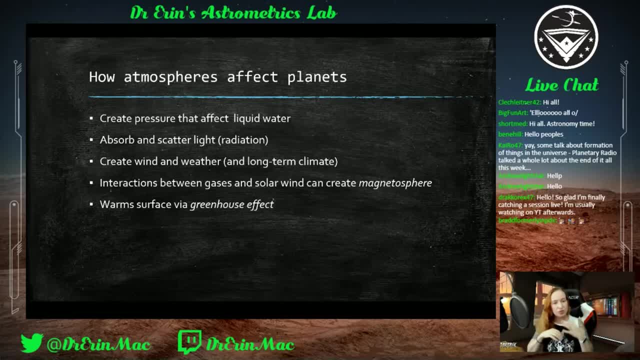 between gases and solar winds that can create a magnetosphere. So think more about the fact like this one's kind of hard to wrap our heads around, but think about the northern and southern lights. That's now. that's not strictly magnetosphere. 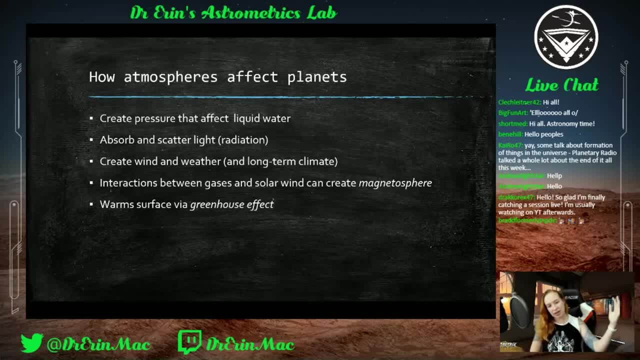 But this is kind of the same phenomenon: that a solar wind hits our magnetic field. Okay, That's a separate thing. but that solar wind then follows the magnetic field up to the north or south poles and then hits the atmosphere, And that's the part we care about here- Once it hits the atmosphere. 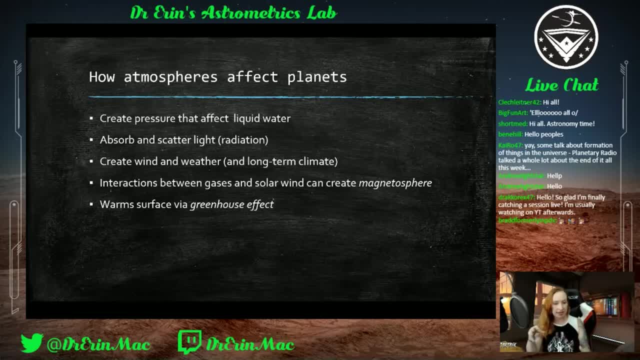 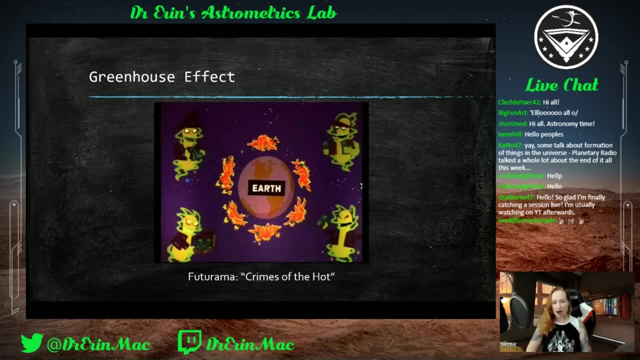 it ionizes and it gives off some light, And that light is the northern or southern light. So that's that interaction that we get there, And then the atmosphere warms the surface through the greenhouse of. you, I hope, have heard of the greenhouse effect before, but if you haven't, again. 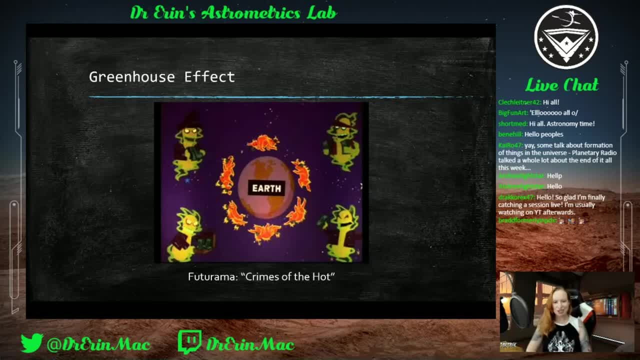 because I really don't want any of this taken down for licensing issues. otherwise I would have played the clip. If we were in a classroom I would have played the clip. But the Futurama episode, Crimes of the Hot, starts out with a great old-timey style science film that explains: 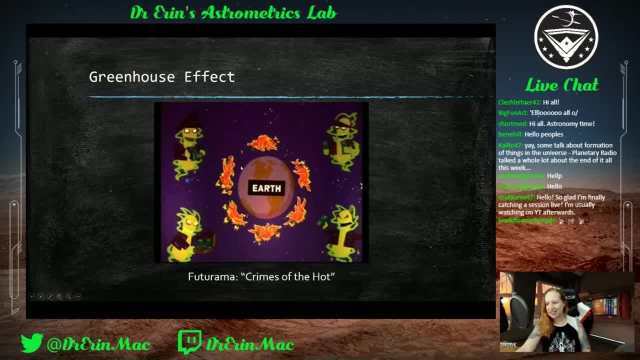 how greenhouse gases work. And the greenhouse gases are these mobster dudes here. And then the sunlight comes in and it's like, oh, this is a greenhouse. And then it's like, oh, this is a. and then when it tries to go on its merry way, it gets beat up by the mobster dudes and the dead. 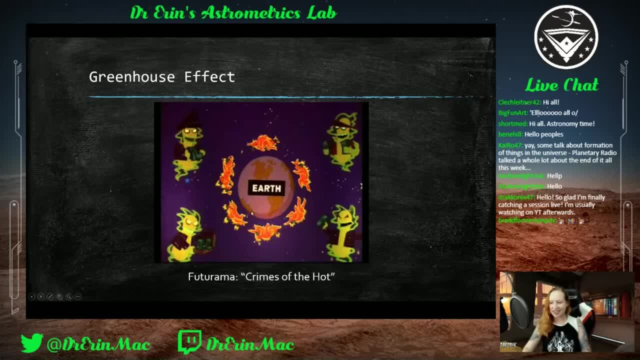 bodies of the solar radiation get trapped around the surface. Now that's a cartoony quick, easy explanation of the greenhouse effect, But what it really is, remember when we- and again I keep saying- remember. if this is your first time here, no worries at all, We've talked about this before. 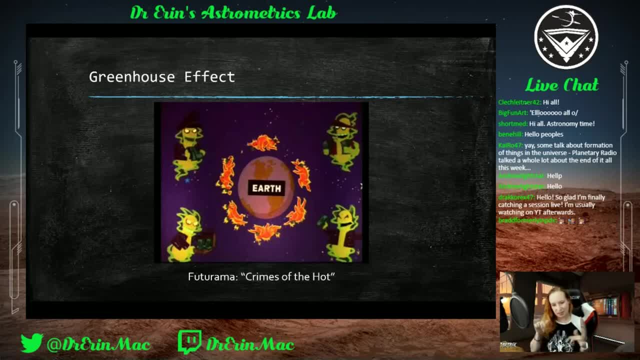 If you're interested in learning more, there are past videos. You can find them on here or on my YouTube channel. But we talked about thermal radiation of planets, the fact that the sun hits planets and then that sunlight gets radiated off, But with greenhouse gases that are present in the atmosphere, what happens is the sunlight. 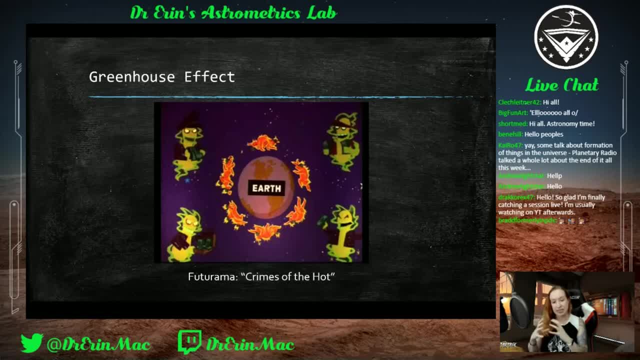 hits the earth and then the earth radiates heat in infrared right. Predator heat gives off radiation. When those infrared photons are trying to leave, greenhouse gases absorb infrared radiation and then rescatter infrared radiation So it's not able to leave And the more greenhouse 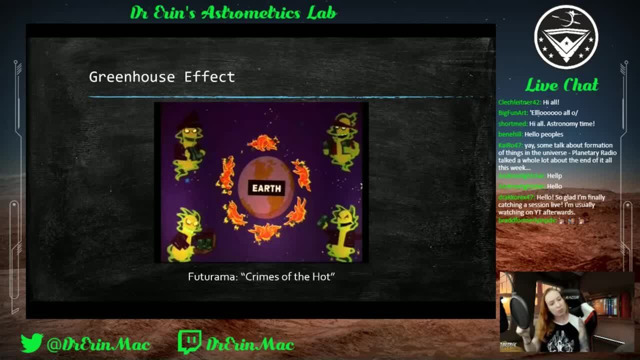 gases you have, the more molecules there are present that will absorb that infrared radiation. So it gets harder and harder for that heat, those infrared particles, to actually leave the atmosphere. If there's a lot of greenhouse gases, it'll just keep absorbing and re-emitting infrared radiation, which is heat, I hope. 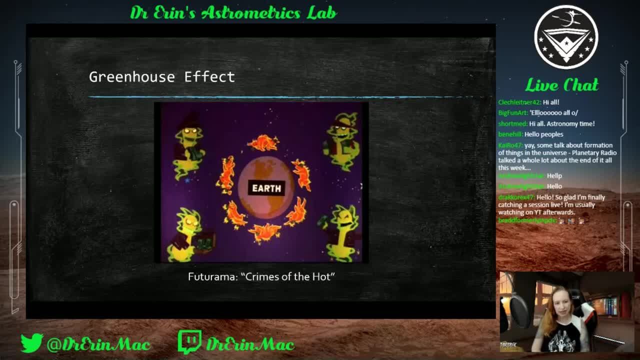 that makes sense. That was one of those things that kind of clicked a little bit later than it should for me, But you know sometimes it takes a while for that sort of stuff to sink in. So that's how greenhouse gases work. They trap and re-radiate heat And, depending 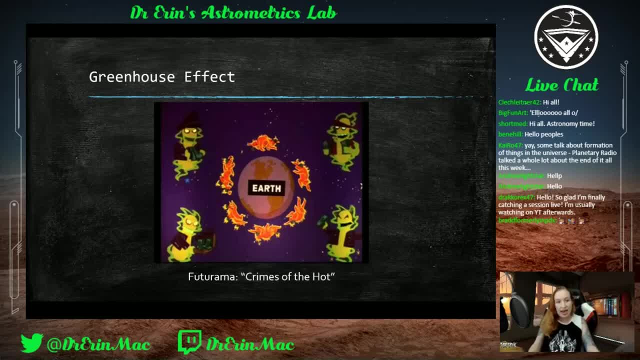 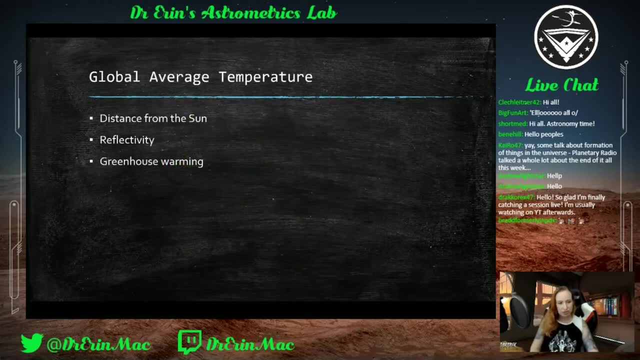 on how much you have in your atmosphere. that will dictate how much of it is trapped. And, yeah, All right. So, talking about the global average temperature, just when we're talking about planets in general, when you're saying, all right, what's the average temperature of this planet? It has. 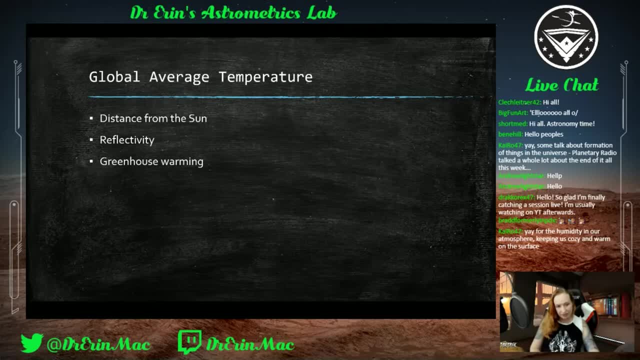 it dictates both from the distance from the sun and the reflectivity, and also the greenhouse warming effect. Yeah, Cairo, Exactly. Humidity in our atmosphere, keeping us cozy and warm. Cozy and warm Sometimes, Right Uh. so the distance from the sun, the sun- right, That's right Yeah. 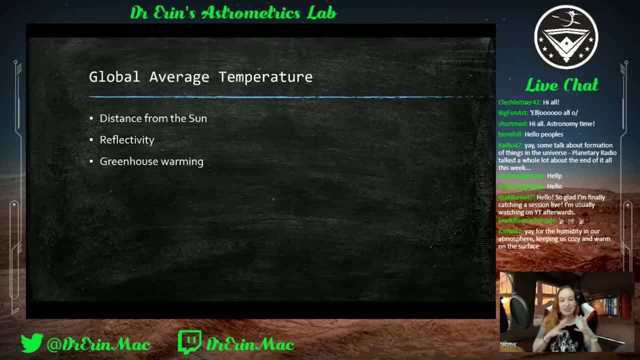 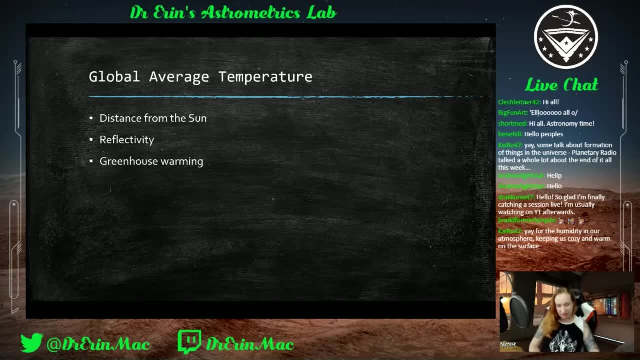 going to be colder the further you are away, And the reflectivity of the planet is also called its albedo. So a high albedo will mean not what you think it means, but mean that it's very, very bright and that it reflects a lot. This really comes into play with, like polar caps, sheets of 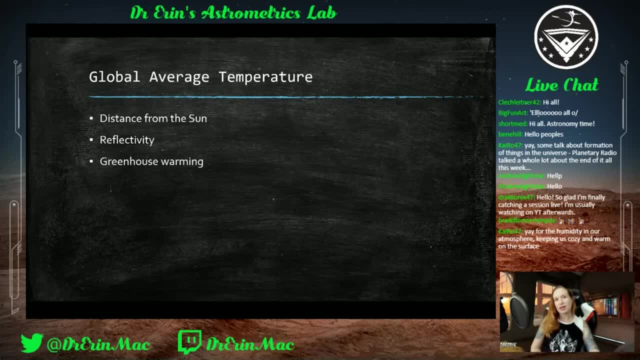 ice, because ice is really reflective And so that when we say it's reflective, that means those photons hit and they bounce right back off again. That's reflected, So it's not absorbed, It's not converted into anything else, It's just reflected off. And so because of that, that affects the. 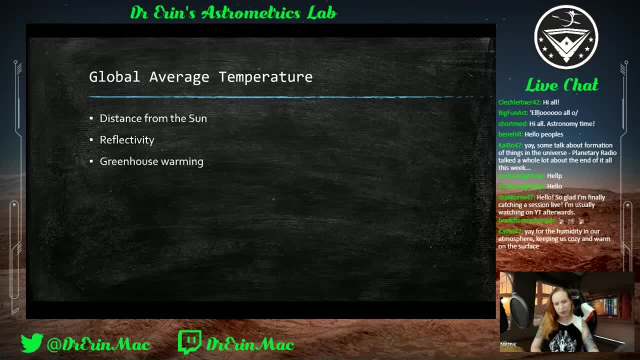 temperature. The more reflective you are, the cooler you're going to be because you're not able to absorb. So equivalent of wearing a white shirt on a sunny day versus a black shirt on a sunny day. you're going to have different reflectivity and that's going to. 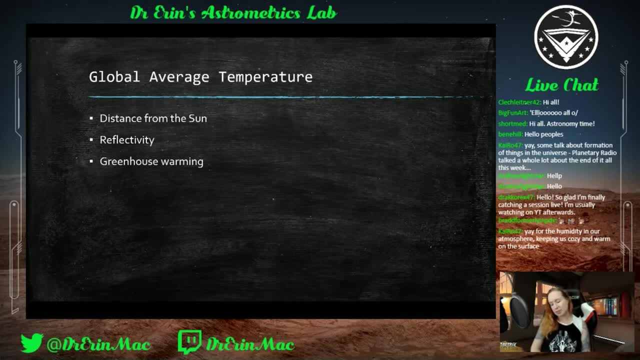 affect the temperature, But the greenhouse warming actually has a big, big impact on the global average temperature, particularly talking about Earth, because, yes, Cairo mentioned we, you know we experience our temperature. here We have some concept of what it is If our, if Earth did not. 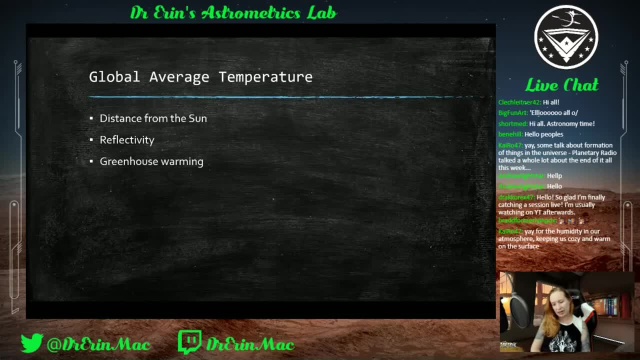 have greenhouse gases and didn't kind of trap its heat a little bit from the atmosphere. if it was just how far away from from the sun we are and just how much we're reflecting, our global average temperature would be just about- I think it's- zero C, I want to say. 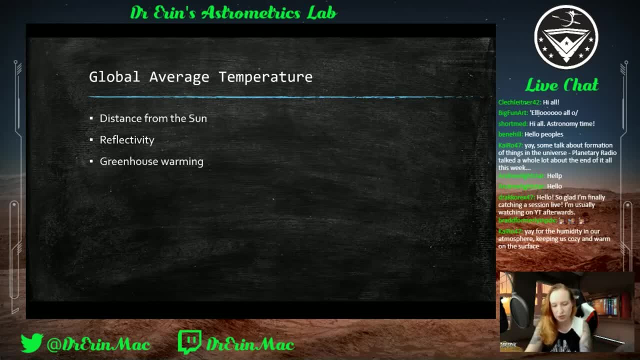 I think it's no zero Fahrenheit, Sorry, So not not freezing water-wise, just freezing person-wise. I would not be comfortable in that. So yeah, it's about zero degrees Fahrenheit. So it's, it's cold, and that's how, what it would be without our atmosphere. 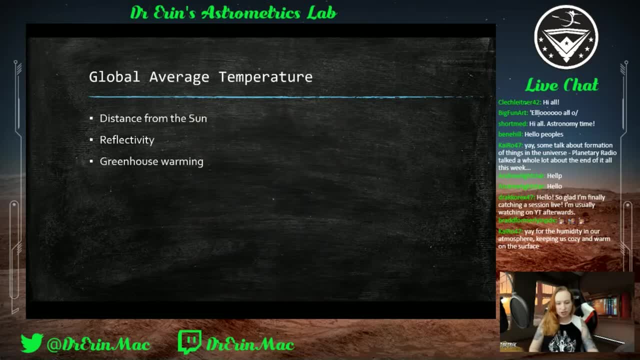 So our atmosphere is good. However, just you know, I'm not. if we did a whole segment on climate change, which I think is important and something that we should all learn about and understand, that would be the entire class today, which is not what I want to do, But it is important. 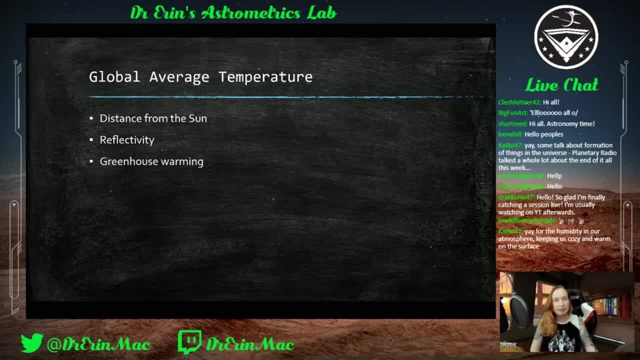 to understand that the increased greenhouse gases are trapping more and more heat and our global temperature is going up and it is caused by humanity and manufacturing and uh, it's irrefutable data on that, So we don't have to get into that debate now. 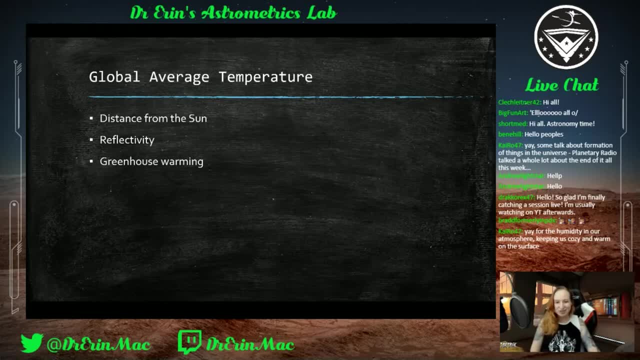 We can get into that debate later if you want. I don't have any. like I said, it could be, I could, we could talk about it for the whole hour and I want to teach some astronomy, but it is important. Please learn about it If you're, if you're curious, and you're really not. 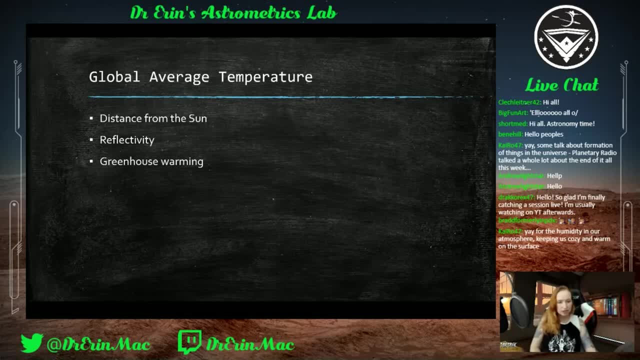 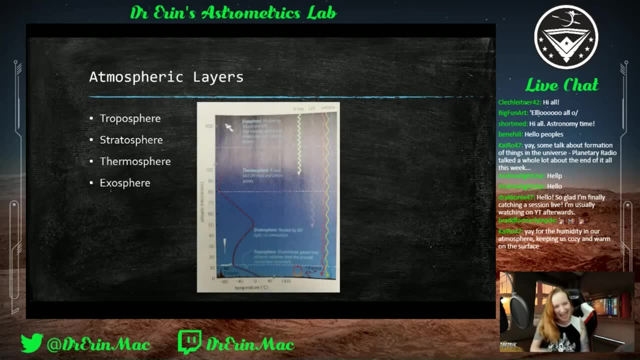 sure, um, reach out, I'd be happy to talk to you about it. Um, I have no problem having those conversations, uh, but I want to teach astronomy right now. So, uh, talking about the atmosphere, I apologize for the picture because, uh, I just took this picture myself. Um, but the atmospheric 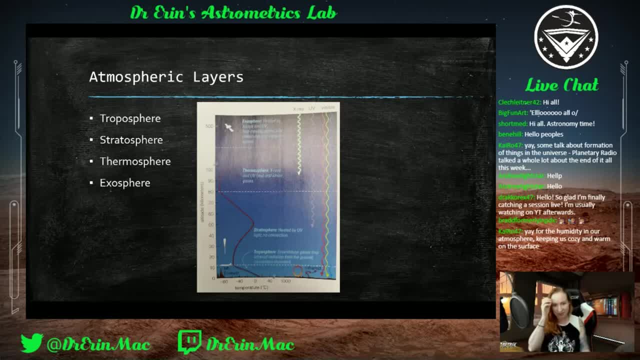 layers as far as we're concerned, at the astronomy level. so this is not like meteorology, atmospheric science discussion level. here We have, uh, these four layers which are then flipped around when we're going bottom up here. So, uh, it's starting from the ground and going up. We have this. 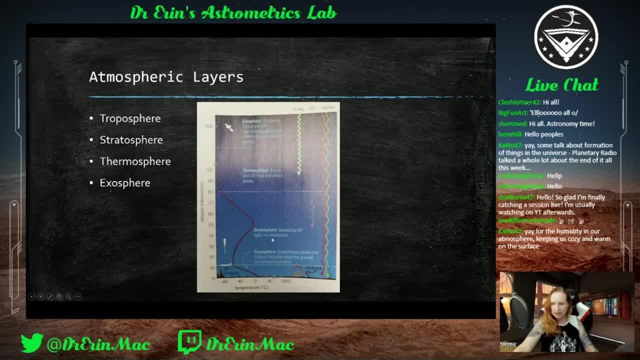 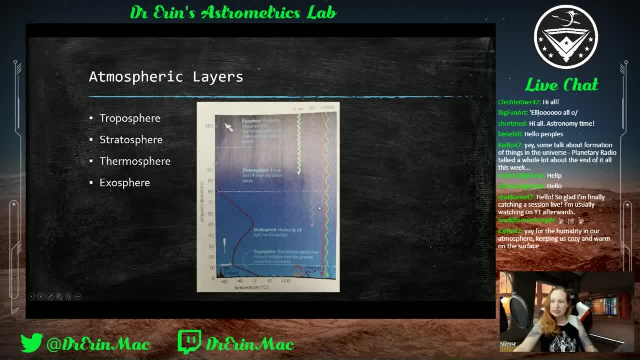 what the temperature gradient is and what electromagnetic spectrum it's absorbing or allowing through. So when we talk about our troposphere- the part down here- this is where greenhouse gases live. Um, and as you get higher in elevation, the temperature decreases And we. 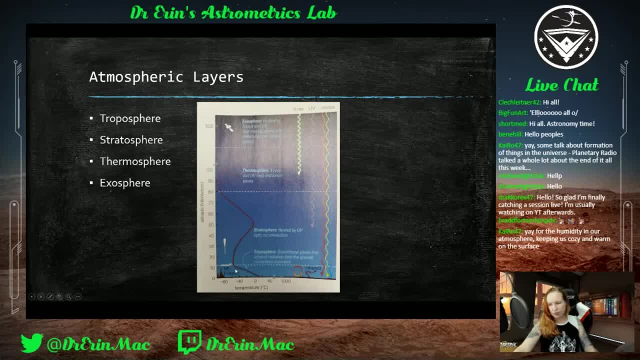 kind of know that intuitively. right, You go hiking. it gets colder as you go further up, Um, and then, as you, uh, transition into the stratosphere. and then this little part here where it seems to make an elbow and go this way. This is also called a mesosphere. 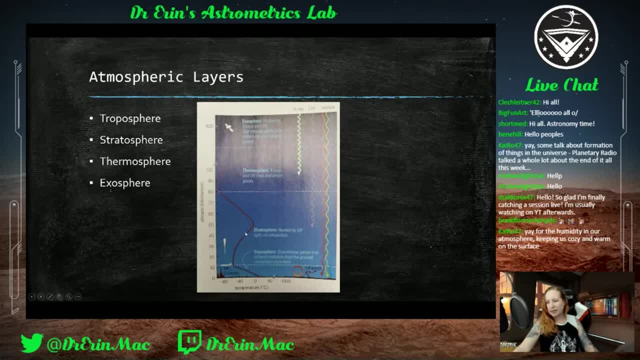 but we're not worried about that, So we're not going to talk about that right now. Um, but the important thing with the stratosphere is that you see that it starts to heat up as you are going further and further up, which is super counterintuitive. 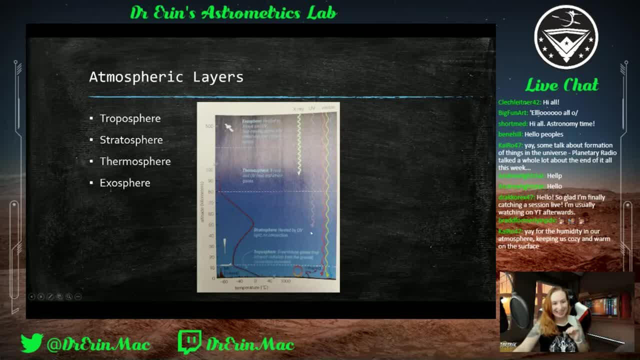 But that's because um the ultraviolet light gets absorbed at the stratosphere level And because we're absorbing this higher energy light, this ultraviolet radiation that's heating up the atmosphere. Another way to think about this. remember that um temperature is based on. 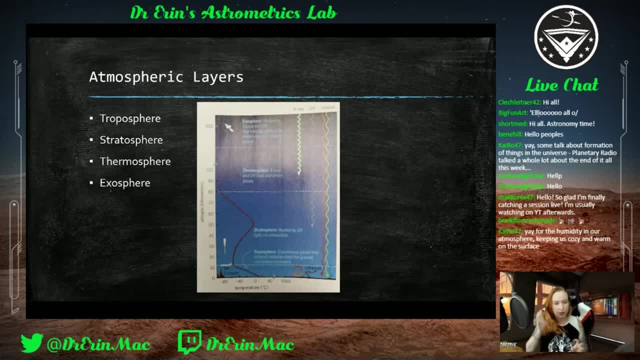 average kinetic energy of particles. This is what we talked about when we did sort of the physics classes. Uh, you take, you go down to sort of the molecular atomic level. that movement and that vibration of those atoms and molecules is what creates that thermal energy. It's really the. 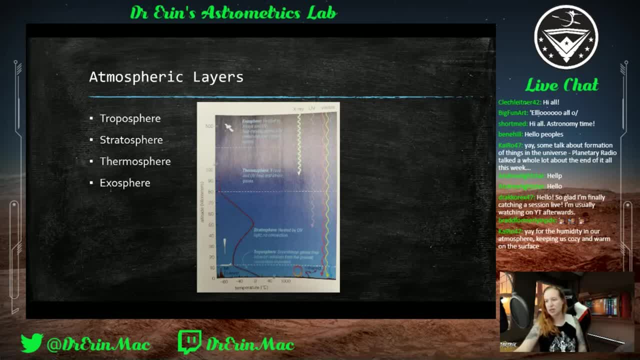 kinetic energy of these molecules just moving around. Um, that's, that's heat. So because we're absorbing ultraviolet radiation here there's more vibration and it's heating up as you go up. Then it starts to transition and cool down where it's not absorbing that ultraviolet. 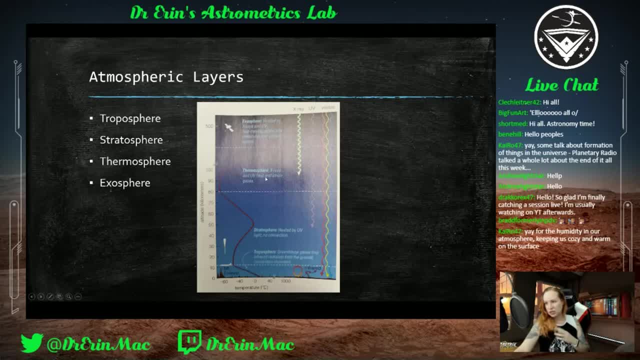 radiation. Then we get to the thermosphere, And so now we have X-rays and ultraviolet heat are are heating up and ionizing gases, So there's even more energy being pumped into this here. So this is where X-rays are mostly absorbed, And then, um, the temperature does start to. 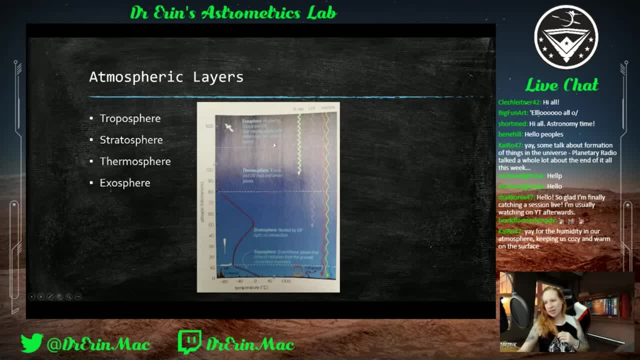 drastically increase the high energy. So this is where the ultraviolet radiation is, And then we get to the exosphere. The exosphere is basically where you're just starting to lose atoms and molecules just because they're so far out. Um, they're still mostly trapped by gravity. 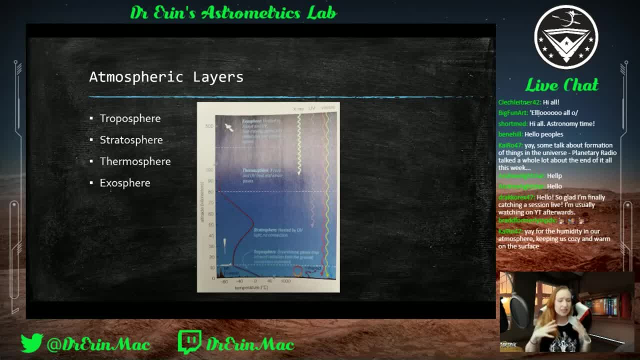 You know, the, the Earth's gravity, the planet's gravity is keeping these atoms and molecules where they are. but it's very easy for them to escape. So, um, if they're fast, if they're heated up, if something happens, they're going to escape. So, um, and then we get to the exosphere. 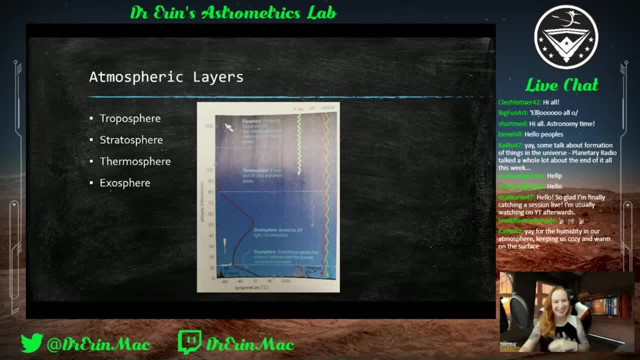 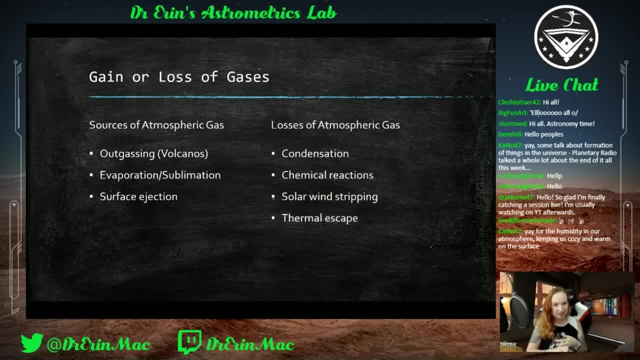 Then they'll fly off, never to be seen again, And we'll talk about that process here. So the gain: how atmospheres can gain or lose gases- And it's okay to get really giggly here, because outgassing is still one of my favorite things ever- Um, I had to do an entire satellite discrepancy. 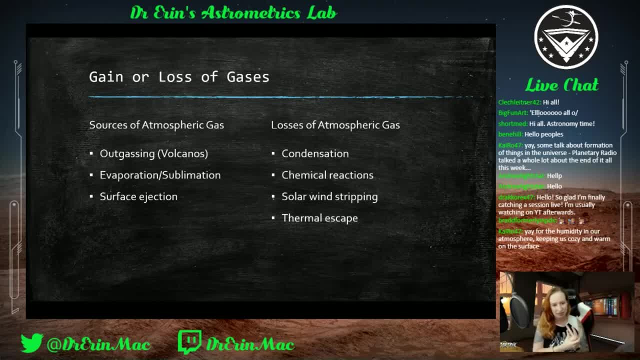 report one time on unexpected outgassing and I could not make it through the day without giggling. So it's okay to have an immature sense of humor sometimes. Um so, sources of atmospheric gas, exactly, uh, sources of atmospheric gas. how we add atmosphere is um, through outgassing. 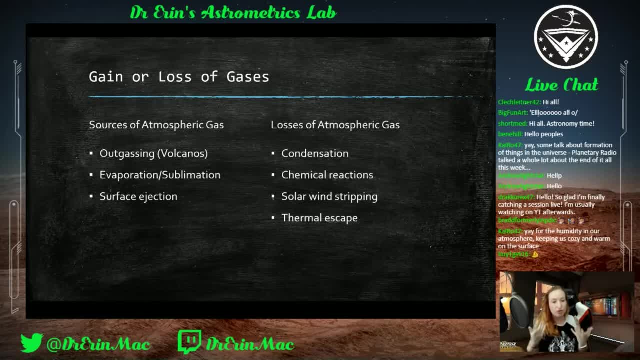 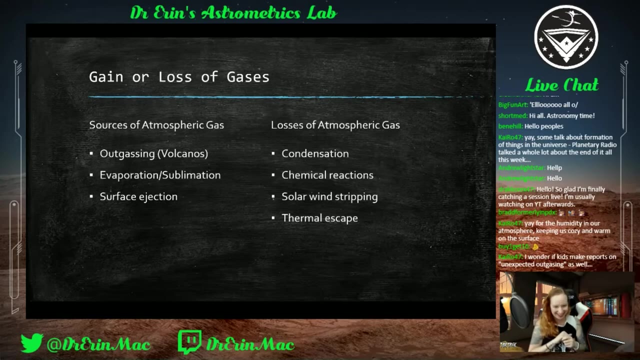 but through the um, through volcanism, right, Letting gases that are trapped under the surface go out of the surface. I highly recommend you start using outgassing in your everyday language, because it's hilarious and it's fine, So I highly recommend it. Um, I think it's funny. 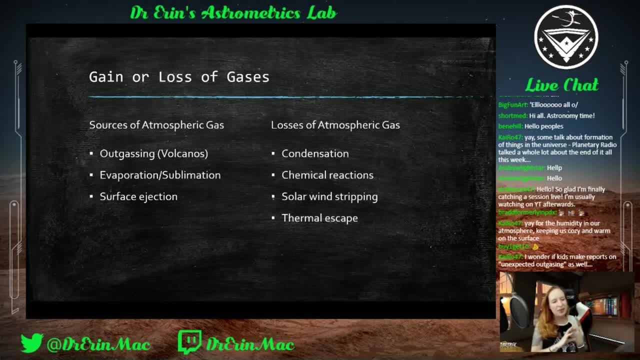 but I think it's more fun to use outgassing than uranus. I'll just put it that way, Okay, And then, uh, we get evaporation and sublimation. So this is, uh, you know, ices just evaporating. 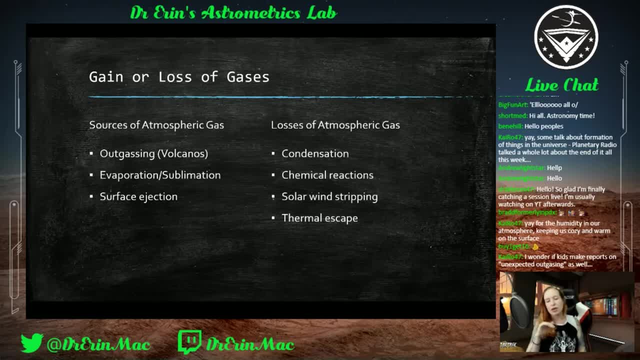 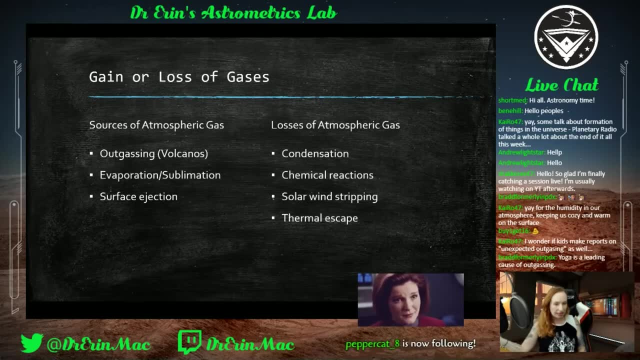 Sublimation is where you go from a solid directly to a gas. So sometimes, when light hits ices that will, instead of melting them and going through the liquid phase, they'll turn directly into gas, And that's what sublimation is. And then the liquid to gas phase is evaporation. 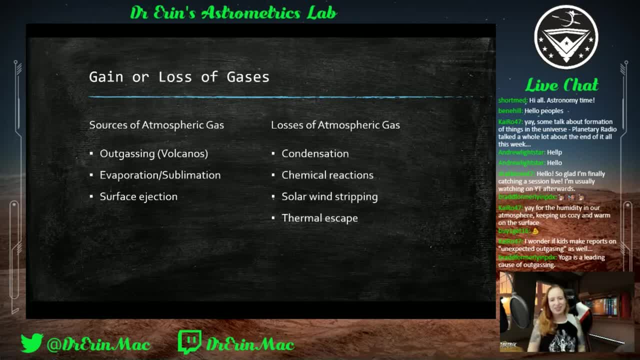 And thank you for the follow, Peppercat, Happy to have you here. Thanks, Brad. Yoga is a leading cause of outgassing, You're not wrong? Uh, and then surface ejection. Um, this is when, like things hit the surface. And so, for example, if you- and this is kind of 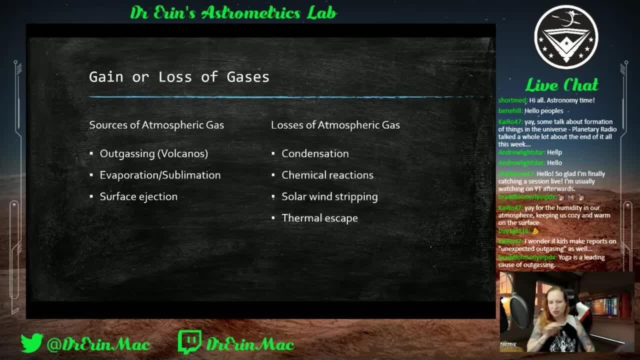 talking more about the other um terrestrial planets, not so much Earth, because we have such a relatively thick atmosphere, Not a lot of stuff can make it through to do this. But if we're talking about Mercury and Moon, when um meteors hit the surface, that will eject material. 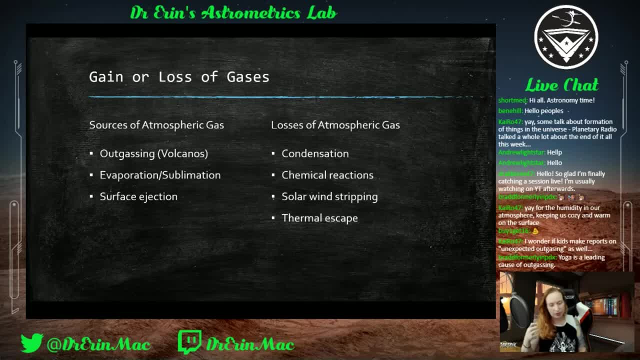 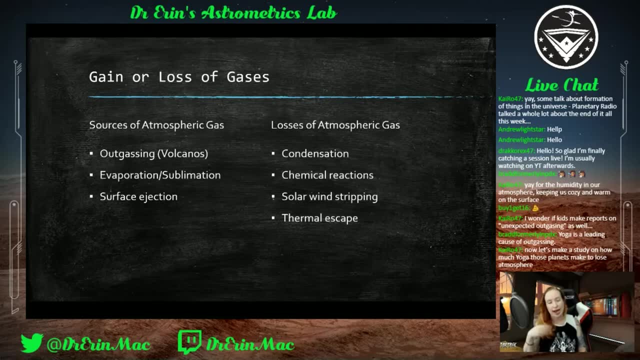 And sometimes that energy can split apart the molecules, Sometimes it can expose pockets underneath the surface, And that's what that surface ejection is. That's starting to add more stuff into the atmosphere, And well isn't, I mean, that's literally okay for those of you? 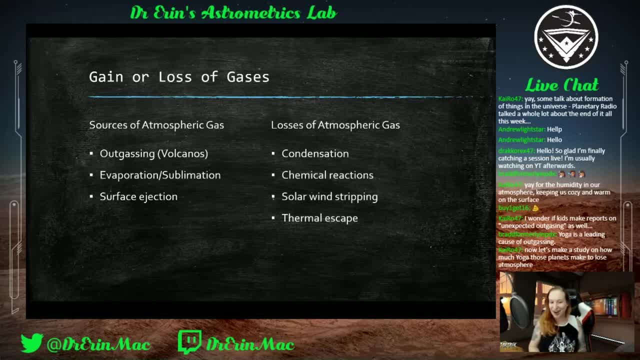 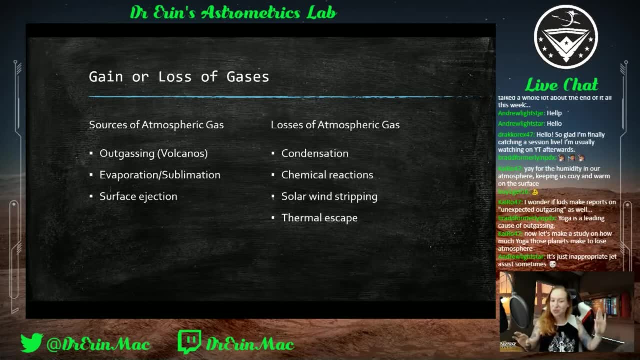 who haven't seen the episode. watch that Futurama Crimes of the Hot episode, Because all of this I mean when I taught Astronomy 101, we just watched the entire episode Because it was like the Earth was getting too hot. They have to figure out ways to move Robots. 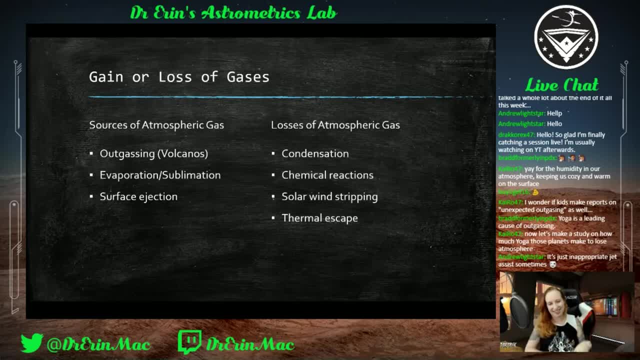 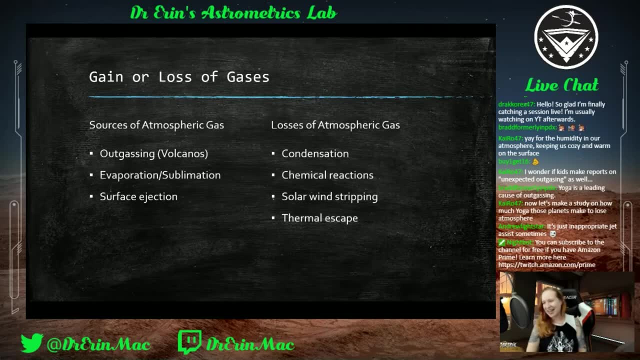 give out a lot of gas. They all out gas in a certain- it's hilarious, Okay, Inappropriate- genesis. I like that too. Okay, So let's talk now about how you can lose atmospheric gas Condensation. Remember that's the phase transition going from gas to a liquid form, um, or a solid. 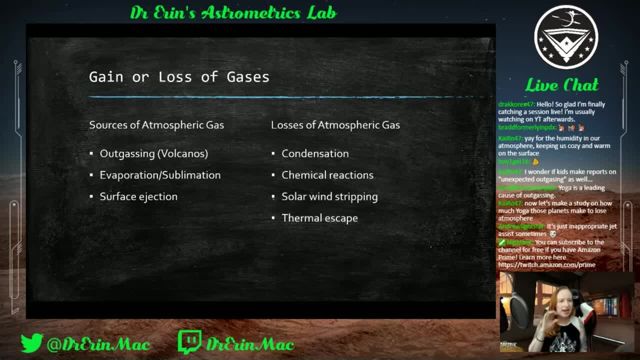 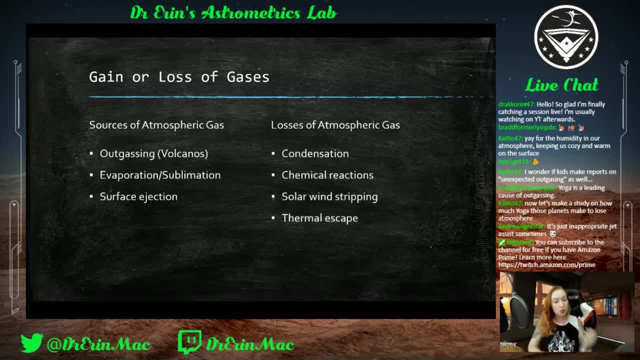 molecules that will no longer be gas form. Um, solar wind stripping. So this is, if the, as the solar wind is hitting our planet, it basically brushes off particles, And that's kind of where you're talking more in the exosphere side of things. Um, and then just thermal escape. Um, 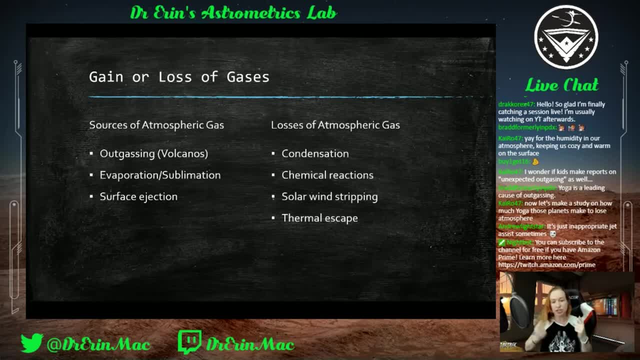 they're, they're heated up and they get more kinetic energy and they take off. So that's kind of again the exosphere side of things. Um, and then just thermal escape, Um, and then just exosphere type type range where um, just because of their motion, if they're heated up, 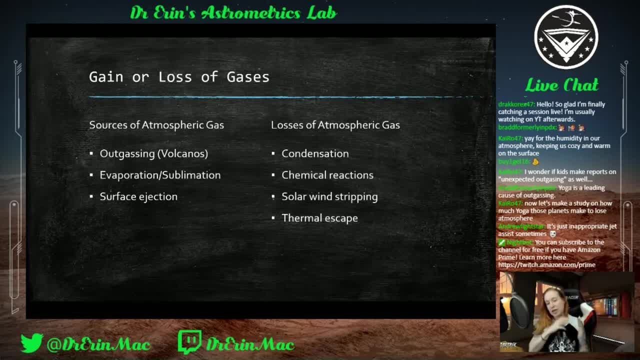 they're moving, So they have some temperature and then that motion, if it's high enough that they're able to escape the gravitational pull of the planet. that's what we call thermal escape. So those are the ways that an atmosphere can gain or lose gas. Let's start talking now specifically. 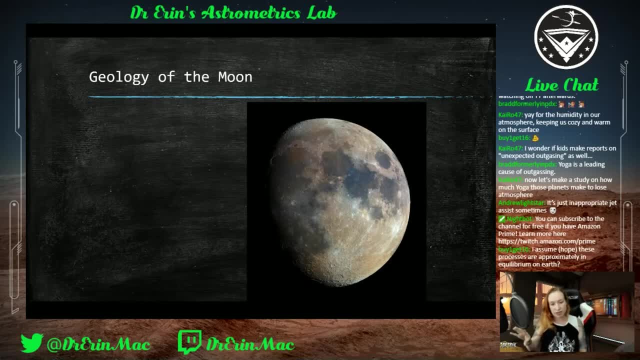 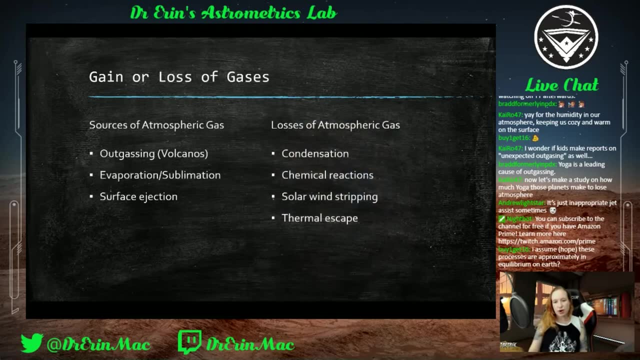 about the geology and atmosphere of the different objects in our, in the inner part of our solar system. Um, by wind, get 16.. Yes, So are these processes approximately an equilibrium on earth? I would say yes, And approximately an equilibrium for most systems that will, um that have a stable 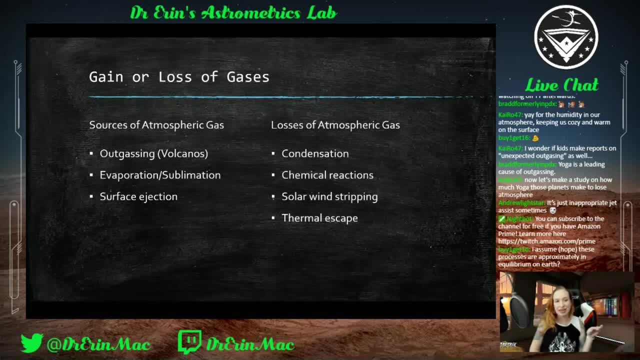 atmosphere. So I say stable atmosphere. So that's things like you know, when we talk about studying planets that are losing atmosphere at a rapid pace or gain, they wouldn't really gain atmosphere at a rapid pace. You mostly would gain atmosphere at a rapid pace or you would lose atmosphere at a rapidате. 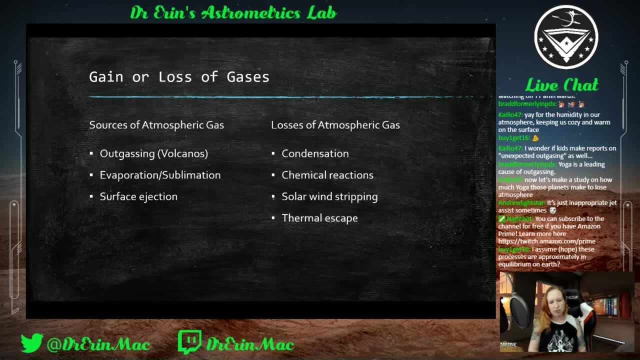 on in the solar system's formation. But once you reach that stability- whereas, like right now, you know our planet's been around for four billion years with the rest of the solar system- we have some level of equilibrium here that we've settled on. But as the atmosphere starts to heat up, those 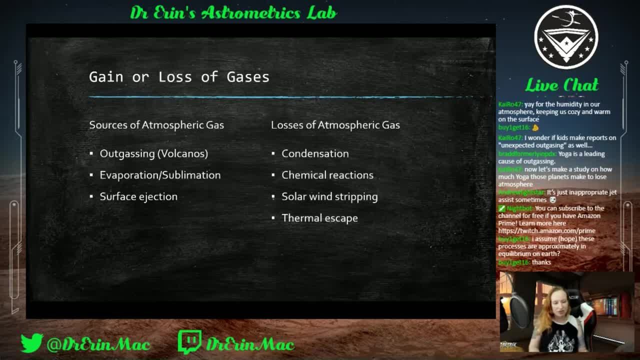 processes will change. Again, it's a little bit of a timescale too. that is hard for us to wrap our head around. In astronomy, you know saying like oh yeah, I mean we're trending toward losing our atmosphere, for example- Not saying that. 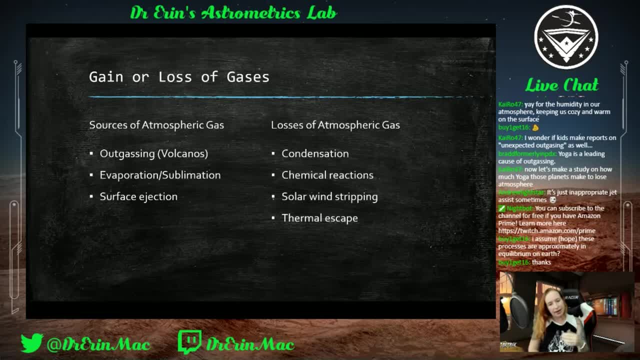 we are, because I don't know what the numbers are exactly, but that could be hundreds of thousands of years, right, So for us it doesn't necessarily matter that much. But, yeah, thanks for the question. Okay, so remember, last week we 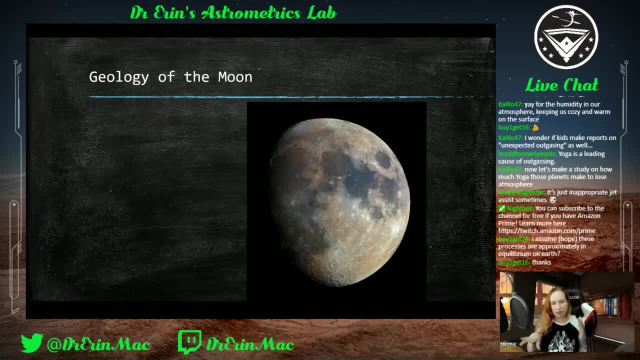 talked a little bit about just general geology and I'll kind of come back and reference some of it here. I'm gonna go and talk about the Moon, Mercury Mars and Venus, and we're gonna talk about the Moon, Mercury, Mars and Venus and we're 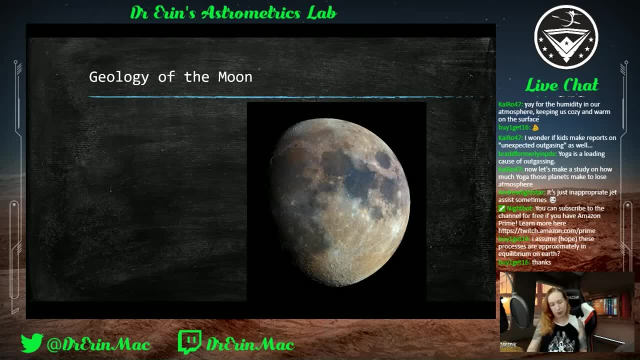 gonna do, the geology and the atmosphere of them both as we go through. So this is a very, very, very pretty picture of the Moon. We like it. This is the near side of the Moon, But talking about how they formed. So these are what we. 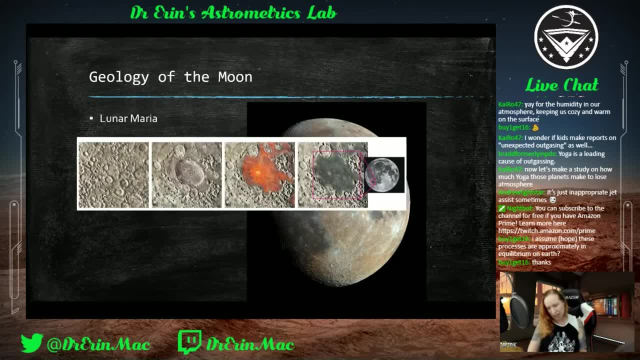 call mare, or basically seeds Seeds, not seeds Seeds, And this is a great depiction of how they form, how they look, the way that they do, And lunar maria, that's it. So here we have basically a projection, not 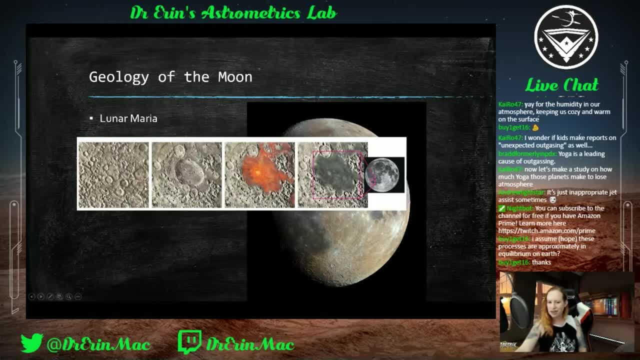 projection progression. It's been a week. All right progression through time. We have this surface here, It gets hit, It gets bombarded, We get a big crater. When that crater happens, remember sometimes we can expose parts beneath and it's. 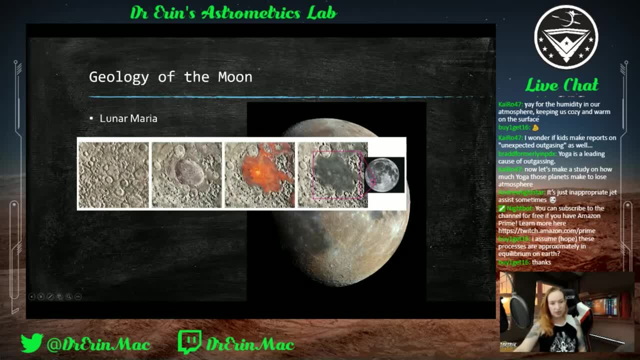 also heated up, because we have this big impact that's transferred some energy, So it heats up, then it becomes molten and then, when it cools off, you get left with this sort of magma-type rock that's left behind, And that is primarily from these. 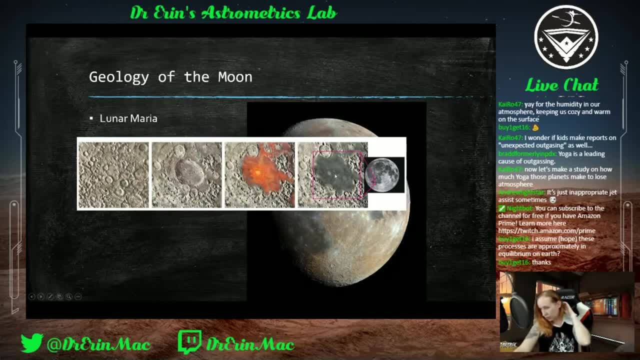 impact craters. So what we see? the lunar maria, especially recent ones like these ones that don't have any craters on top of them. right, You can just look at this image and kind of age every portion of it separately. right, You can say down. 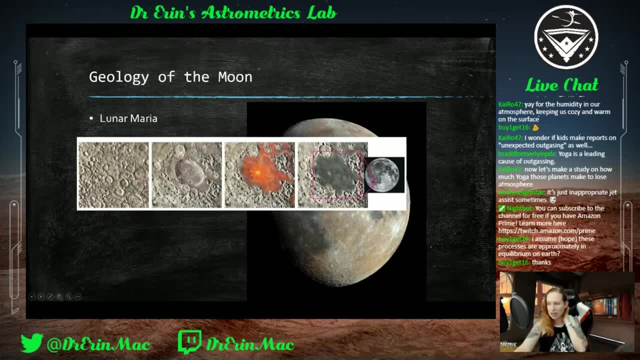 here is the oldest, Here is younger And here is younger here, because this got hit by a crater after this had already formed. So there's different like things you can do with that. That's planetary geology. A lot of that is this sort of detective work to. 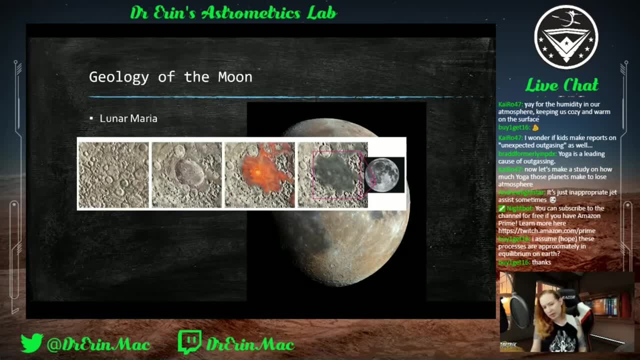 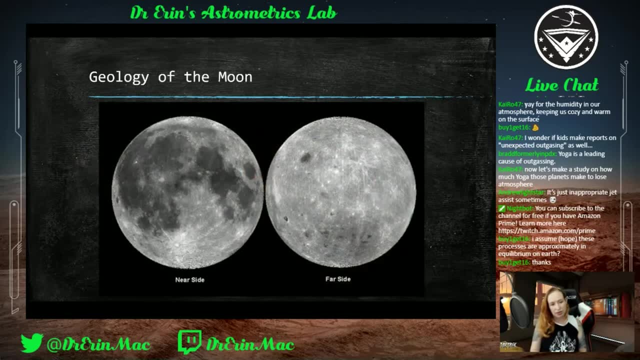 piece this information together, But some of you may have heard the term, and I just used it here- the near side of the Moon versus the far side of the Moon. The key with the Moon is that it's tidally locked with us. So what that means is as: 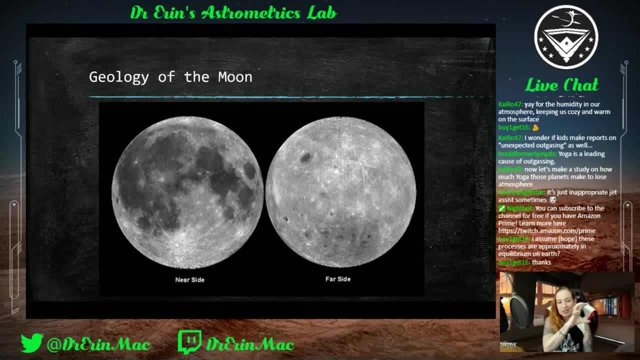 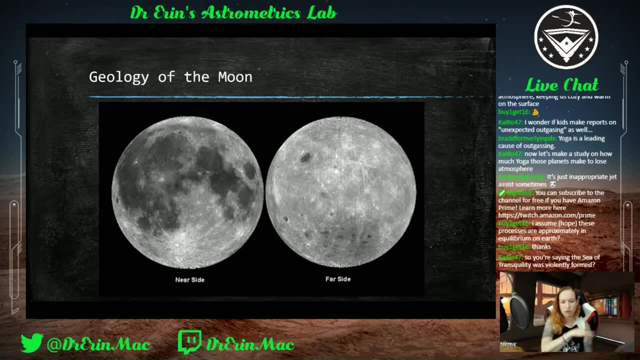 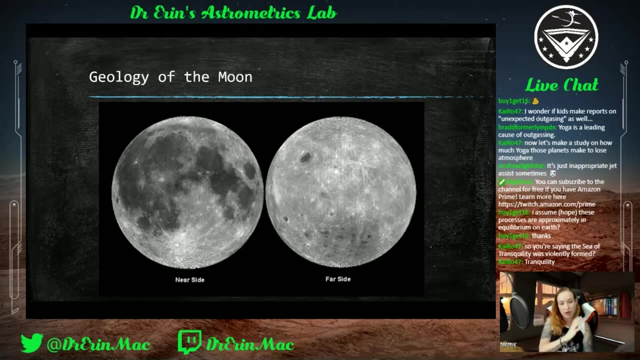 the Moon goes around the Earth. the same side faces us The whole time. This has nothing to do with the phases. We- I mean, if you remember, like 10 weeks ago- we talked about the phases of the Moon and how that's caused by the different angles that the Sun is hitting it at. So 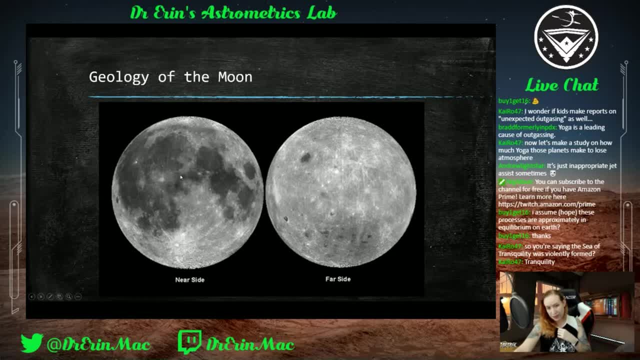 that just determines what part is in shadow, But the side itself that's facing us is always this side. It's tidally locked. Before I continue with that, Cairo is asking: is the Sea of Tranquility violently formed? I mean, 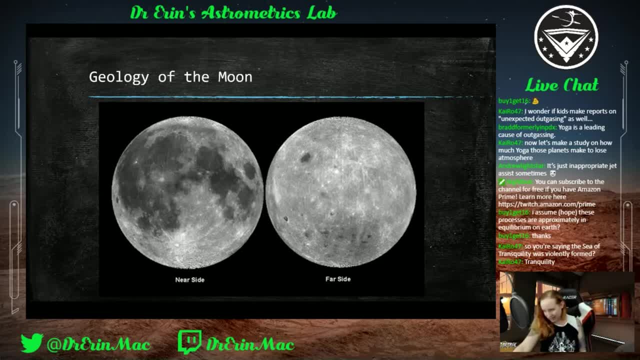 that's an excellent point And I don't know specifically about the Sea of Tranquility, but um, but I do like that comparison and I would say I would say yes. But the big question here is like, okay, if we were just talking about like 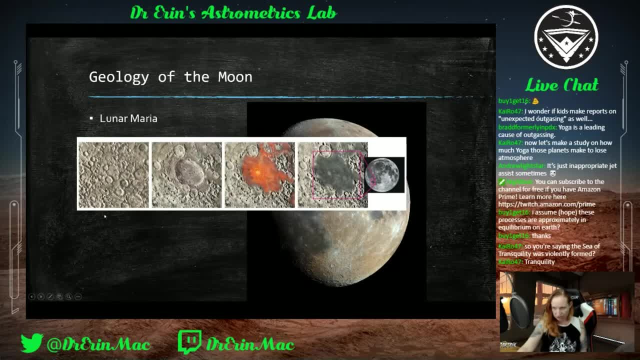 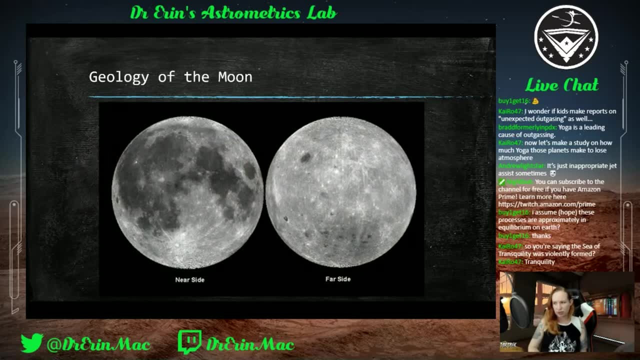 this right, that you have this sort of nondescript surface with a lot of crater impacts, And then over time, it starts to look like this: why don't the both sides look the same way? Now, you can still see over here on the far side of the Moon and this: 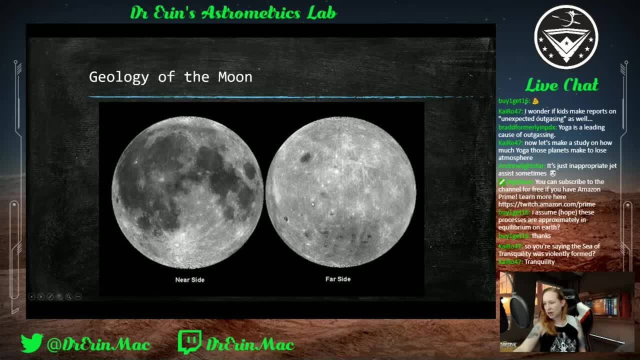 is done through imaging, so this is not a picture taken from Earth, because we never see this side of the Moon from Earth. You can actually kind of- if you're able to see the resolution on your screen- you can actually see these strips that built up this image. 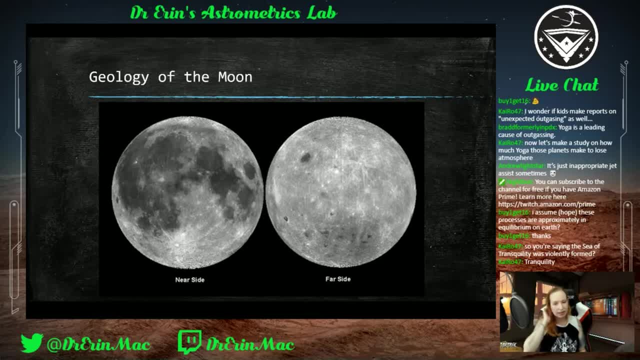 as the imager was rotating, orbiting around the Moon. Aw, thank you for the follow, Quintus, But this far side of the Moon still has some of those, uh, those, um, those seas. God, where did they go? Maria, whew, that's my, that's my word- mental block for the day, apparently. 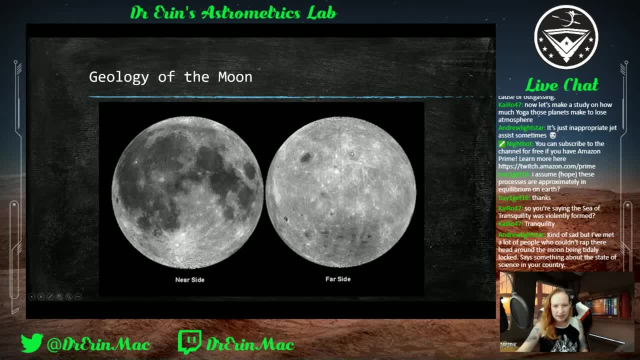 Uh, it still has some of that Maria there And uh, yeah, I mean Andrew, it's you're. it is hard to wrap our minds around. I think that there's a lot of things in astronomy that are still difficult to just conceptualize because it's counterintuitive. 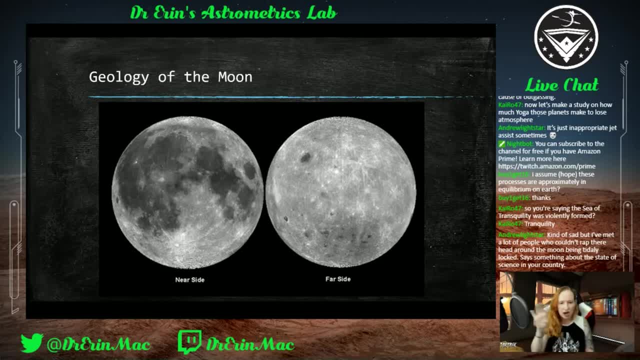 Yeah, And so the idea that it's tidally locked is kind of hard to image and you just kind of have to do this. And then I've seen some great demonstrations where you know you can look top down, and I think we showed this back in my um where we talked about the 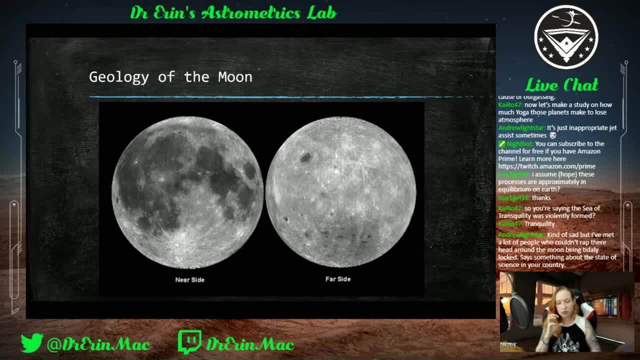 phases of the Moon, where you can see that the Moon itself is rotating and it's just the way that it's rotating around the Earth. it matches its orbit, Um, but the question is, why does it do that And why does the near-circuit? 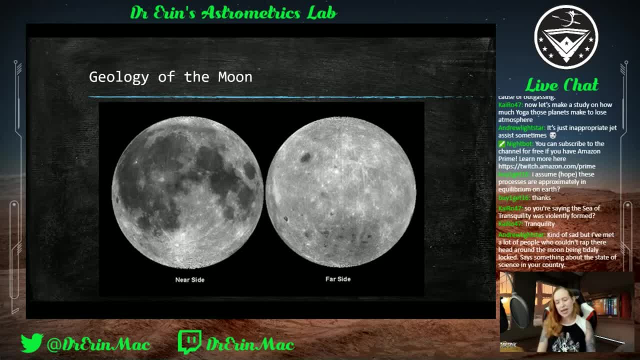 Why does the near-side look so much different than the far-side? And a lot of that has to do with how the Moon formed, how we think it formed, And we've talked about this a couple times, especially a couple weeks ago when we talked about the. 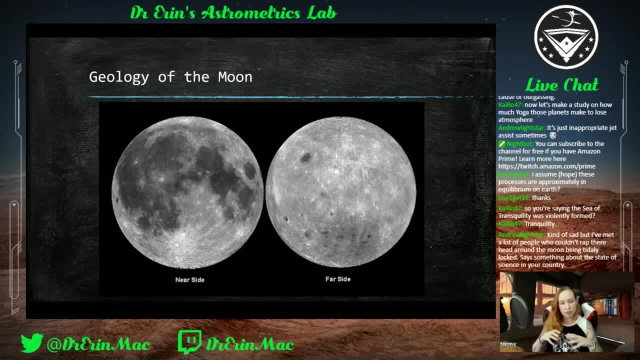 um formation of our solar system, But the idea of how the Moon formed, particularly because it's such a unique object. it's so much bigger and relative to the size of the Earth, You know like it's. if you think Mercury and Venus don't have moons, Mars and 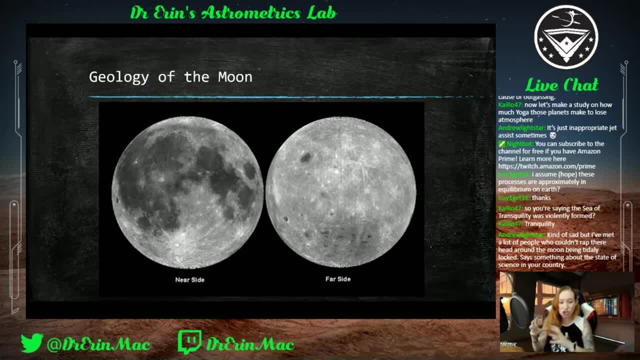 Jupiter have two tiny potato-shaped moons. Earth has this huge honkin' moon around it. So the idea is that early in the solar system formation, where we were starting to get these planetoid things forming, Earth was forming and it was coalescing and it was grabbing. 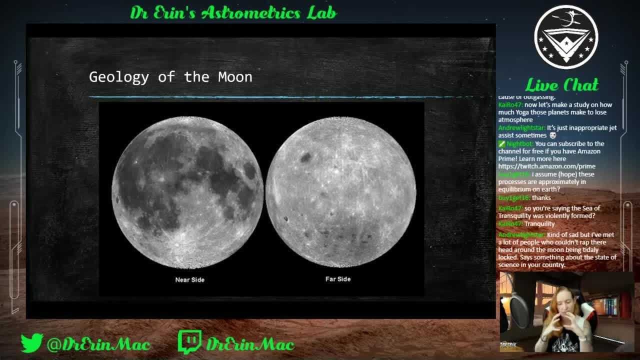 a lot of stuff as it was going, but it was very hot and dynamic and mostly come together, Um, and then something hit it, And when something hit it, it tore off a chunk. And when it tore off that chunk, that stuff. 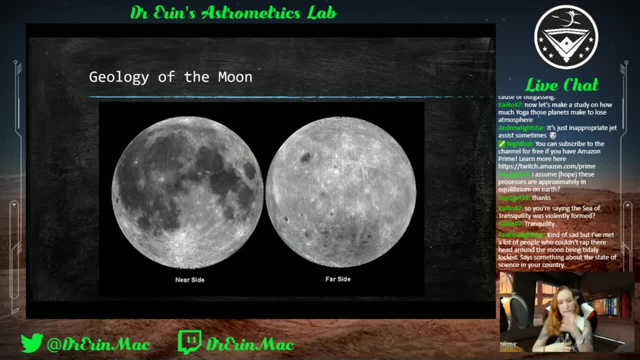 became very dynamic And but it got trapped into the gravitational pull of the original planet, That original planet being Earth, this being the Moon, And because they were both hot and molten, particularly this which had been violently torn away from the parent. 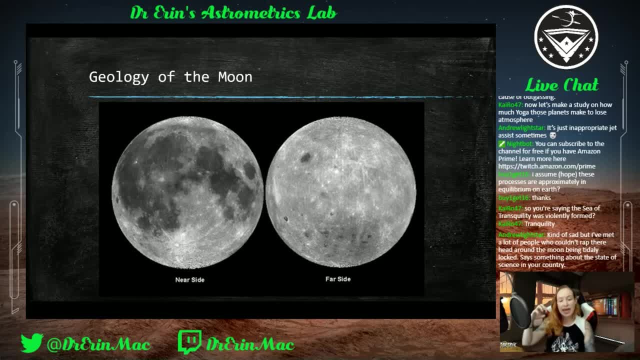 planet. it cooled off, And but as it was cooling off it was pulled toward the Earth. So essentially all that molten magma on the inside was pulled toward the Earth, And so the liquid stuff was more gravitationally distributed towards the Earth than it was. 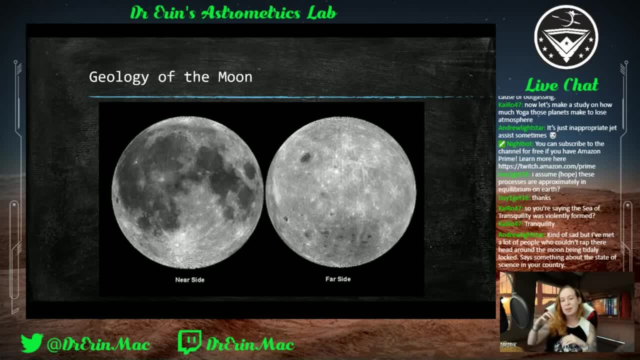 the far side. So all that magma was pulled toward this side And, uh, and then, as it's been exposed, or or even just as it was cooling off, then it solidified on that side. So that's why we have more magma on our side than you do on the other side, because during its formation, 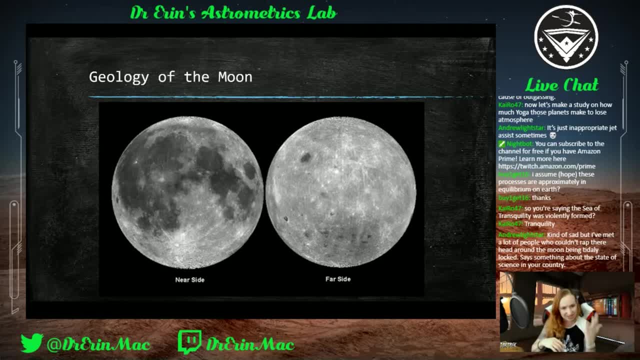 all of that molten magma was pulled towards the Earth's side And that's why it's mostly exposed. I hope that makes sense. Again, this is one of those things that's a little hard to describe in this format, um, where I don't have a classroom that I can jump and dance around in front of in two 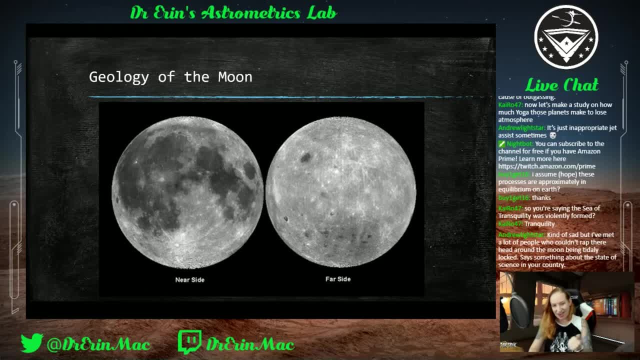 demonstrations. Um, but yeah, so it's important to note the Moon is tidally locked. The same side faces us all of the time And uh, but the tidal locking also, it's not that. uh. that explanation of the formation just explains these, maria. It also explains the tidally. 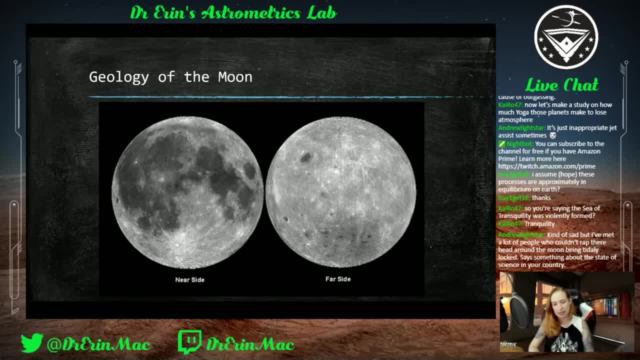 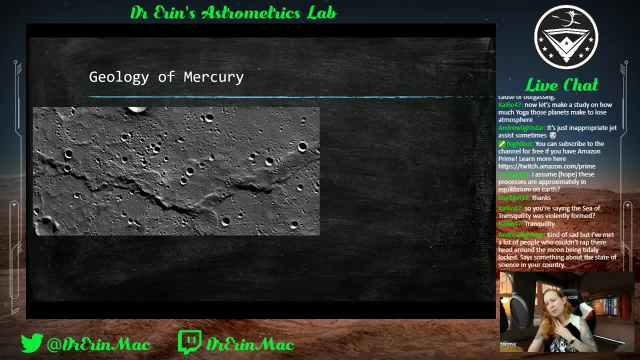 locking why that same face stays facing us the entire time. It has to do with that model of the formation. Okay, So let's go to Mercury a little bit Now. Mercury is weird. Mercury has a very large core compared to its overall radius, If you. 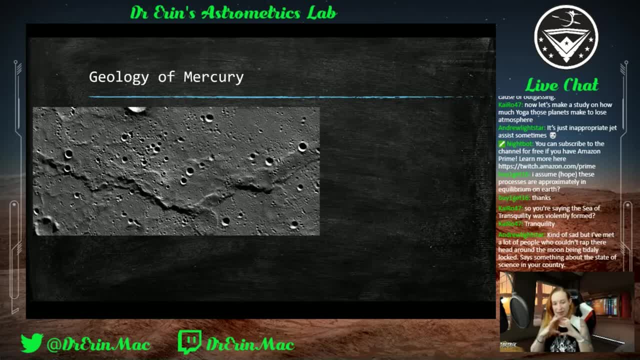 look at the other terrestrial planets, Mercury has got a very, very big core compared to the rest of it. Um, and the thought is is that Mercury has cooled off and it's shrunk as it's cooled off. Now I'm not talking about its distance from the sun, you know getting 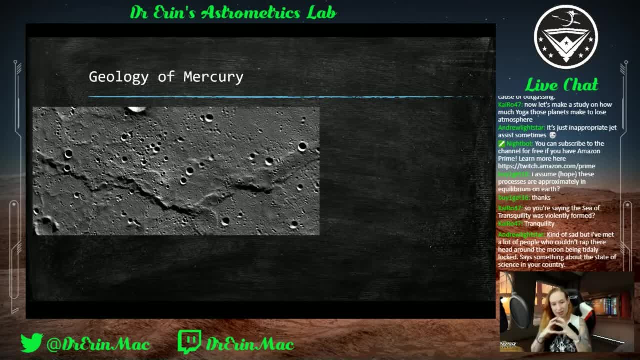 hit and radiated- I'm just talking about the interior of the planet- has cooled off, possibly from some bombarding, possibly just from the size of it. But as it cooled off- this is the cool thing- It's basically formed wrinkles. So I'll try to picture this a little. 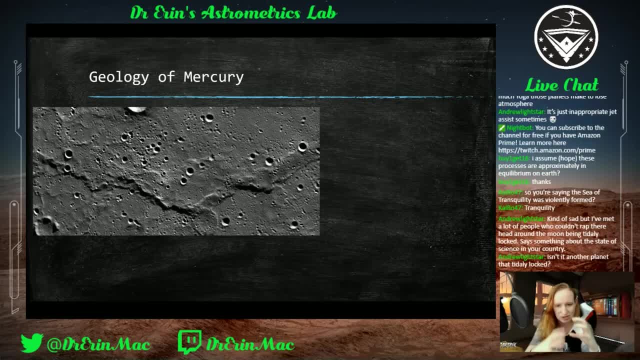 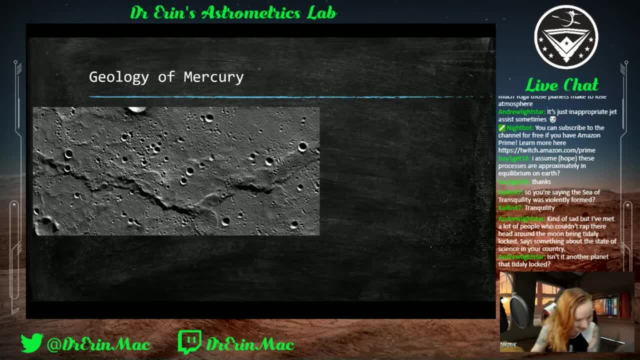 stuck in this side of my head, as it were. Um, I do have any note here, So someone can look it up and just say, is mercury tightly locked? or I can look it up at the end of this Um, but there doesn't seem to be any current sort of tectonic formation that's happening. 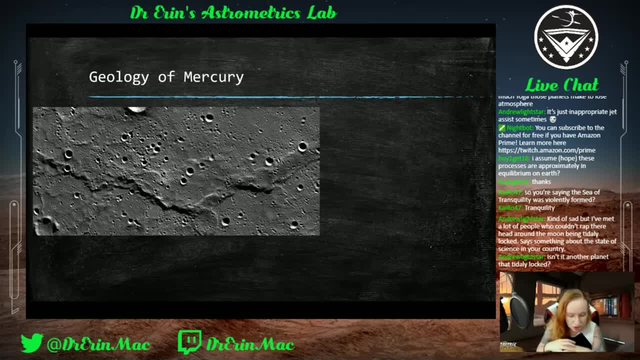 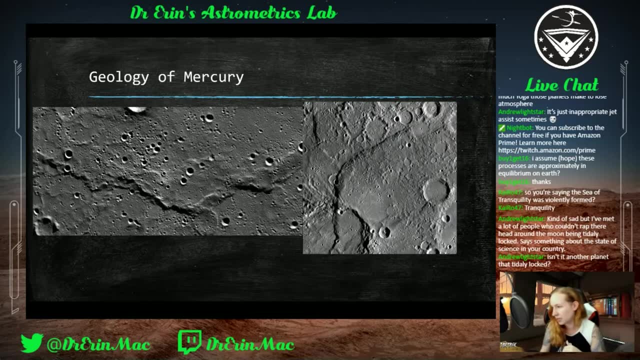 or there's no active volcanism. on mercury, It's just started to cool off, Um, the core in the mantle kind of shrink down and then portions of that crust were forced under each other And that's where you get these like wrinkles on the surface as it cooled off and 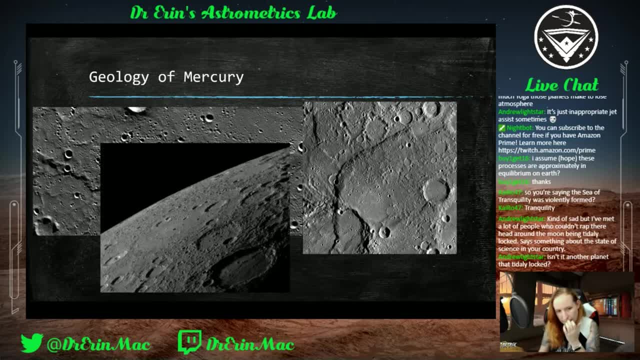 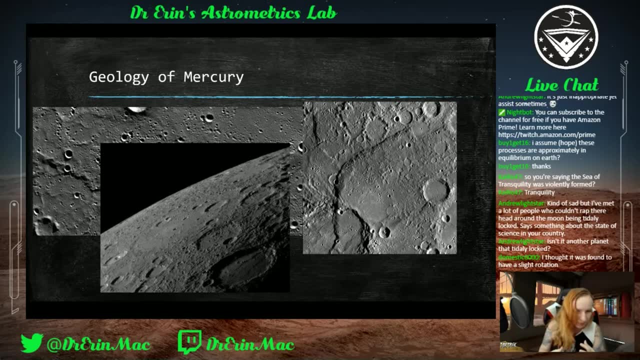 it shrank, which is pretty awesome. And this is just a baller picture of the surface of Mercury, And usually Mercury and the moon are kind of lumped together because they have very little atmosphere. You might be right domestic. Well, we'll confirm that after this, after this. So 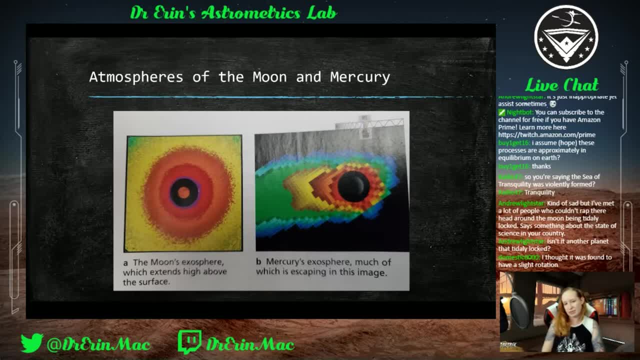 the atmosphere of the two of them. this is like atmosphere, right, It's really just that: exosphere. So remember we talked about the layers of the atmosphere. that very top layer is what we call the exosphere, where particles, if they get enough speed, can just boogie on out of here. 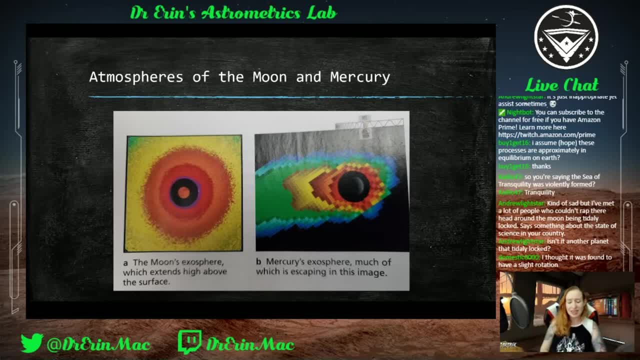 That's pretty much what we have with the moon and Mercury. They have an atmosphere in the sense that there are gas molecules that are trapped in the atmosphere And they're trapped in the atmosphere gravity of these objects, but it's like 0.00001% if that. even that seems like a lot. 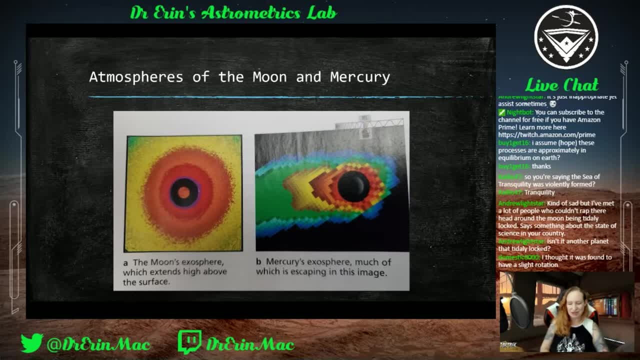 We have this discussion in the discord. I think Todd put in like 12 zeros or something. It's very, very much different, So, but this quote, this image, is really cool. This was another one that I just took out of my book, but these sizes are actually relative to each other. 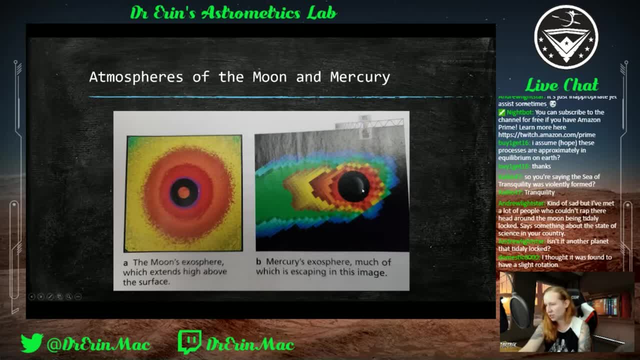 This is the moon and this is Mercury, And that's kind of how big they're compared to each other. And because Mercury is so much closer to the sun, you can actually see that exosphere, all those little particles. It has this structure because the sun is over here and the sun is 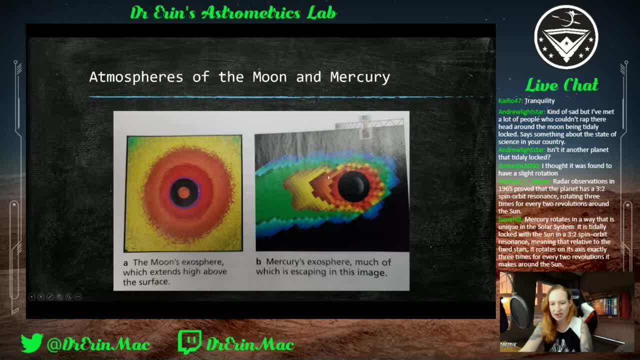 pushing that, those particles off. So you get almost this tail as it's escaping through there. And then the moon is much further away, So it doesn't have that same effect. It might have a little bit of it, but you still have these molecule, individual gas molecules, So it's 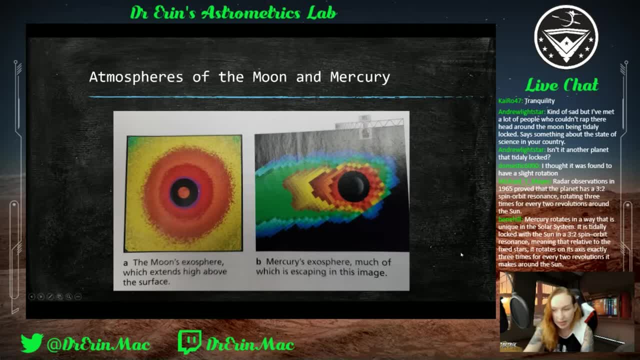 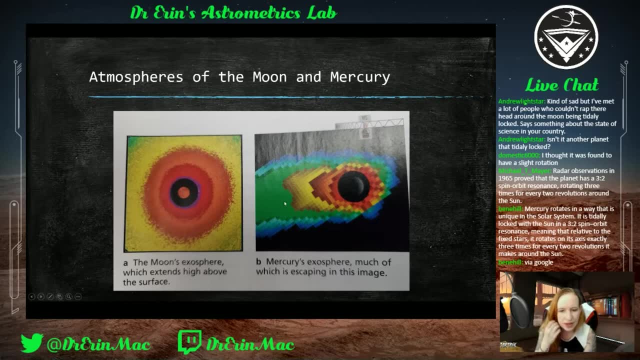 trapped around just gravitationally and they may get enough speed or radiate that thermal radiation escape just so we get here. Thank you, Benny, I appreciate it. Oh, Michael looked it up. Radar observations in 1965 proved that the planet has a three, two spin orbit resonance. 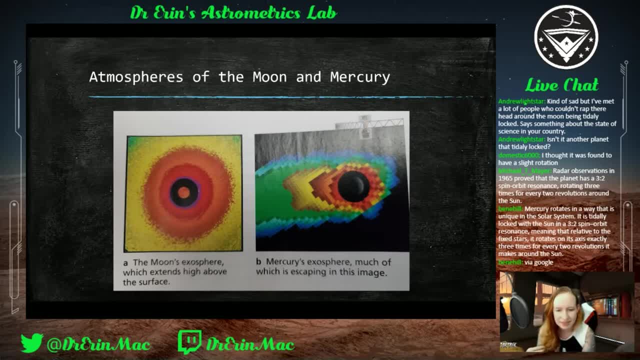 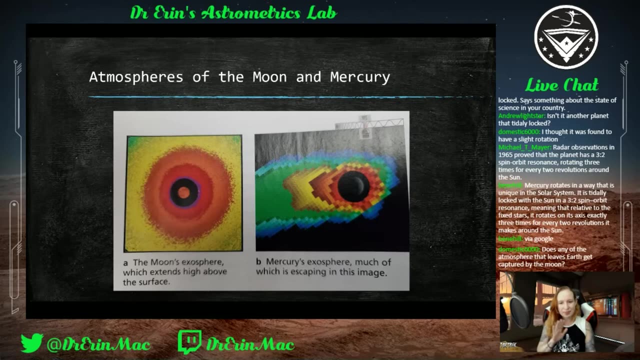 rotating three times for every two. I love resonance, And thank you, Benny. Same thing, Awesome, Relative to the fixed stars. it rotates on its axis three times for every two. resolutions, Math is beautiful, All right. So again, moon and Mercury mostly have their, geology is mostly. 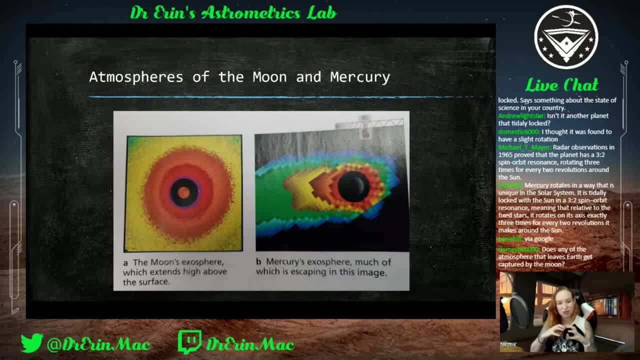 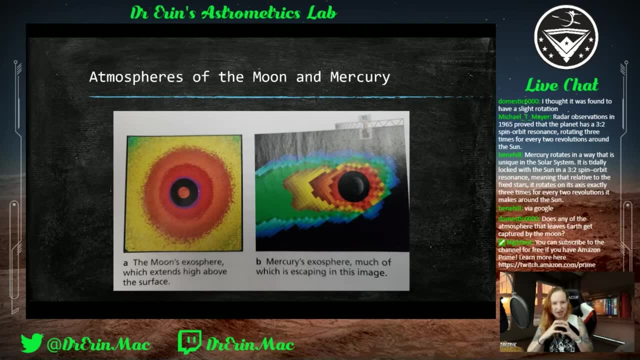 made up of impact craters. at this point, We also have some shrinkage, as George Costanza would appreciate, of Mercury, which has caused these cliff faces, these wrinkles that we get here. Oh, domestic, That's a really good question. Does any of the atmosphere that leaves Earth? 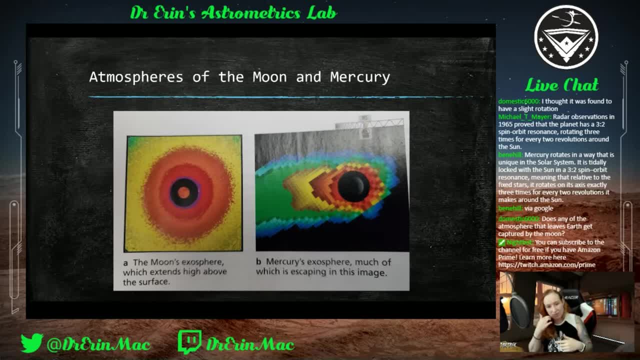 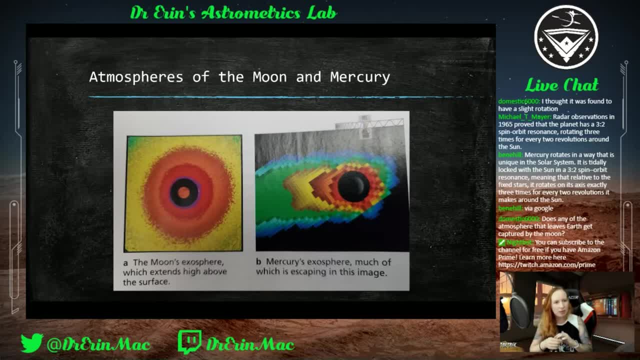 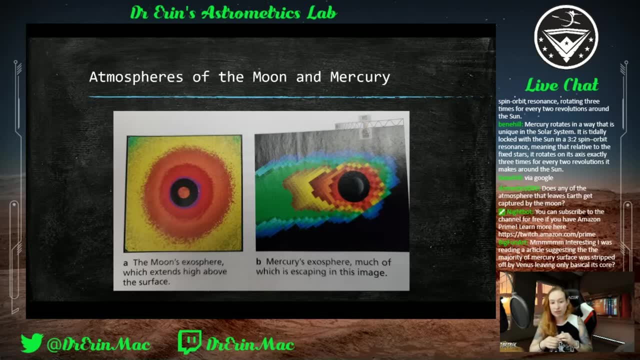 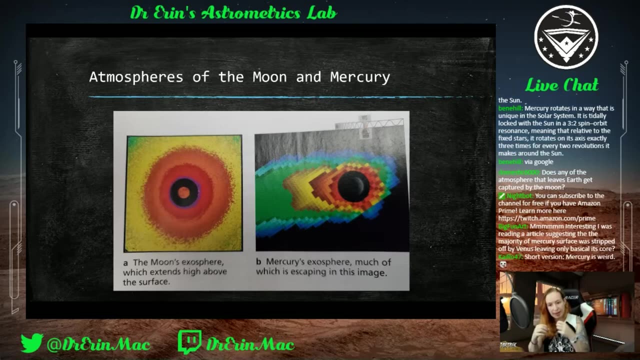 just like there's no reason why it wouldn't. I would probably just err on the side of saying that I wouldn't necessarily claim that most, if not all, of the moon's atmosphere comes from the Earth. I would say it more comes from the impacts that send up gas into the. 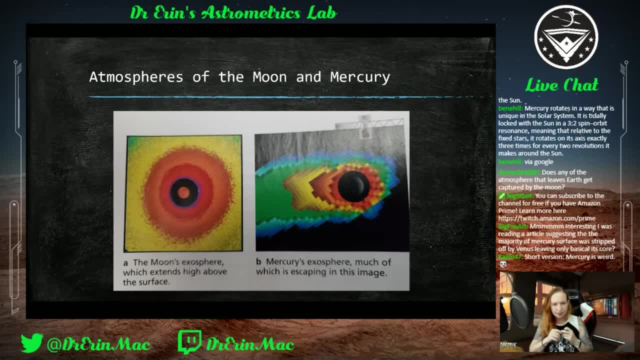 atmosphere. So, oh so, big fun, All right. Okay, Thank you. So the majority of Mercury's surface was stripped off by. so that is, I don't know, I don't know, I don't know, I don't. 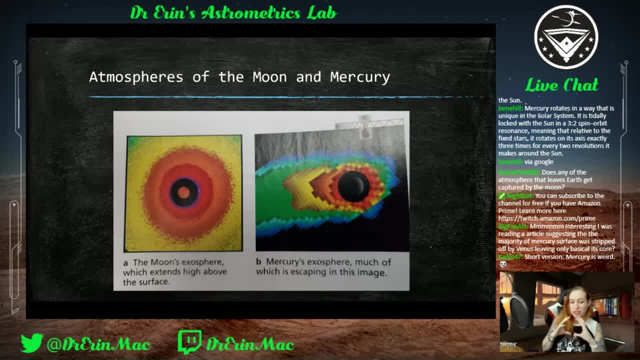 I didn't really go into it that much. That's why we started with a much bigger core relative to the overall radius that during the formation of the solar system. I think that's one of the models. Another model was like maybe that there was just 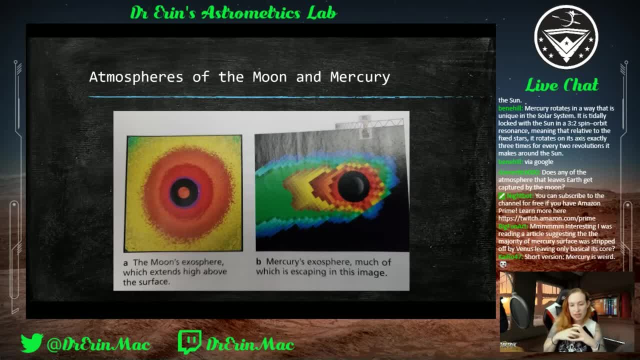 a big impact that stripped off some of the outer layers, But regardless that was more in the formation that just left behind a more massive core. So, again, similarly to how something hit Earth near the final stages of Earth's formation, something hit Mercury, or the gravitational pull of Venus. 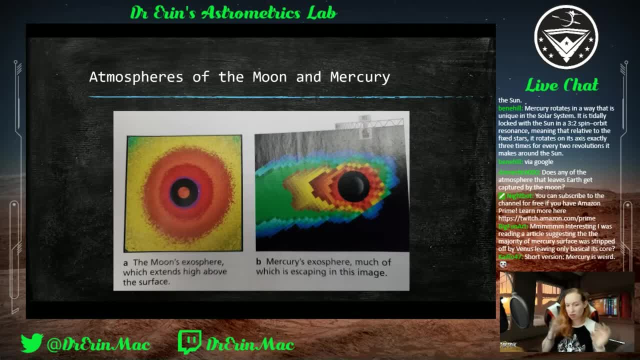 as it was forming and clearing out its orbit, pulled the material off. Both are models for how the core became to be such a big proportion of the radius. Then we go into this explanation of: okay, now that we have that big core. 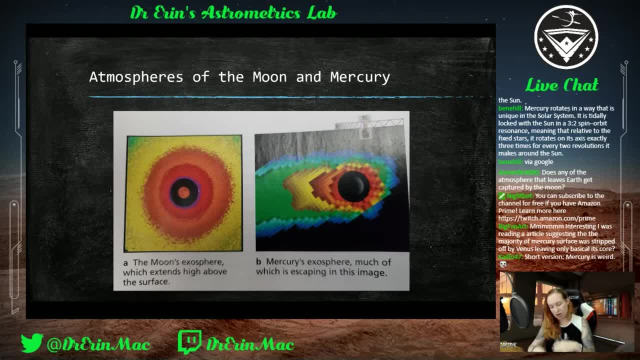 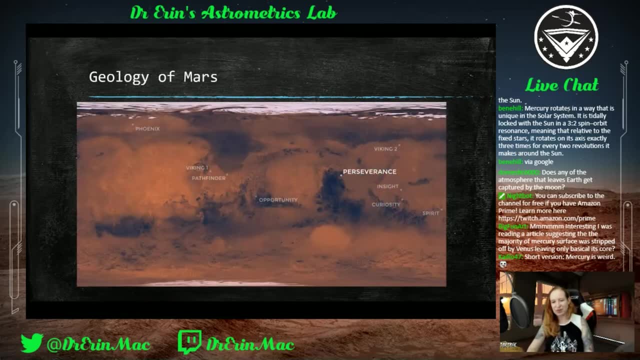 that still is cooling off and it shrank and then caused the shrinkage. Okay, so that's the Moon and Mercury. Ooh, this is. yeah, this is probably gonna go longer than 40 minutes. That's okay, this may end up taking the whole hour. 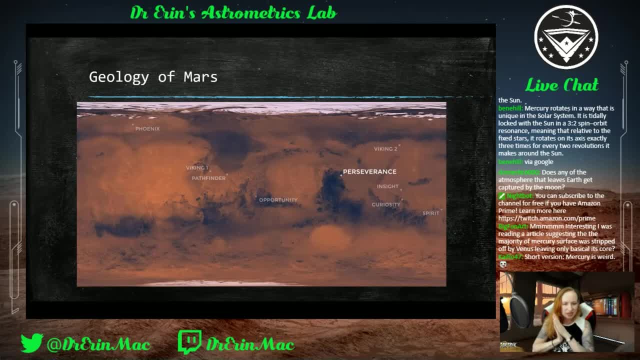 but that's all right, No worries. All right, let's go to Mars. Mars is awesome. I love Mars. This is just kind of a cool layout, flat map showing where we've sent little robots to go check out areas And you can see where Perseverance is gonna go. 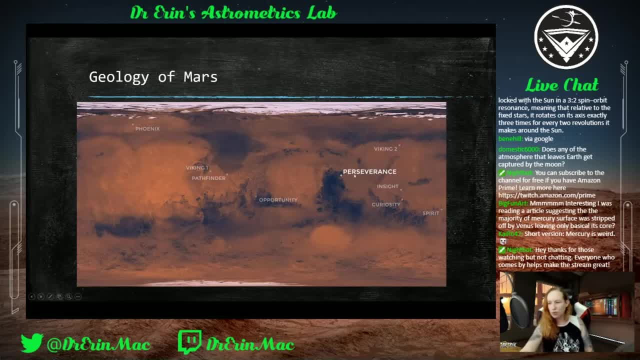 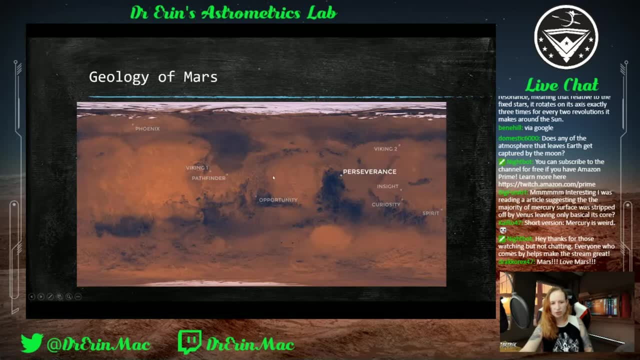 and where all the other two objects have gone, And I think, regardless- if I mean opportunity, we've lost contact with it- may just be established. It's establishing its own mutant territory, robotic colony in this section of Mars, So just be prepared for that. 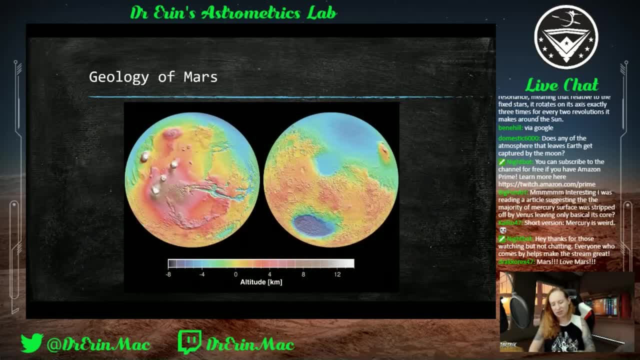 Okay, that's a really old. that's a deep reference to an XKCD comic about how the fact opportunity lasted so much longer than it was supposed to and it ends up colonizing like most of Mars. So I love the geology of Mars. 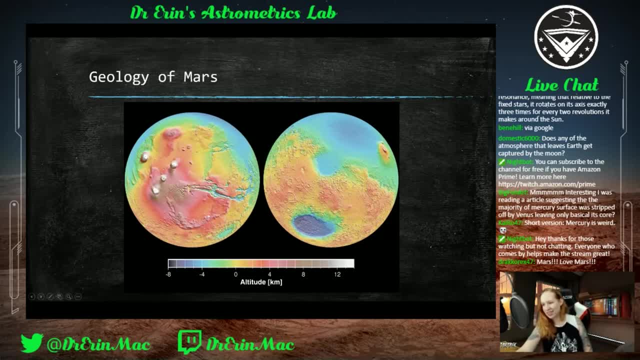 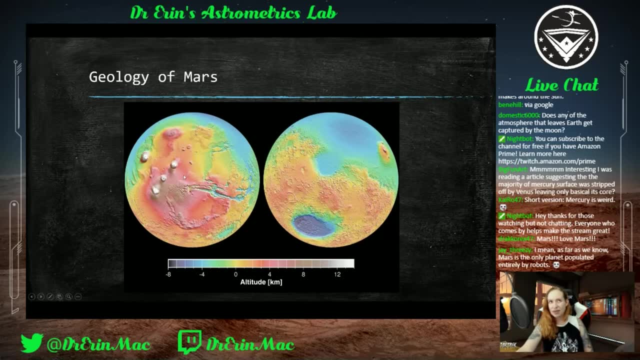 We're gonna come back to like what this hot nonsense is. but the big, big, the features of Mars- Oh, J3Z, thank you, are this one? Hellas Planitia? Then over here we have the. if this was a class, I would have us all say it out loud: 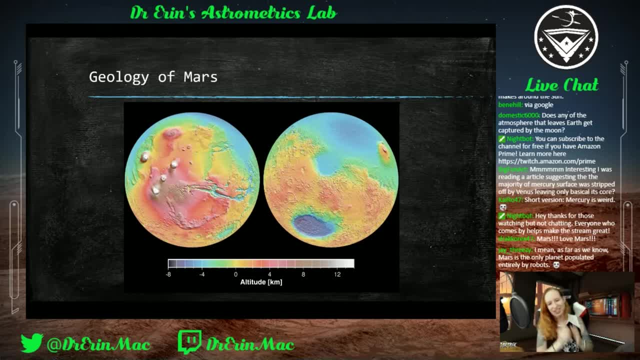 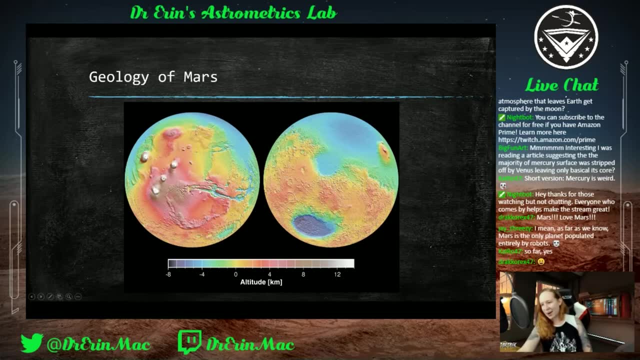 Ready Three, two, one: the Tharsis Bulge Cause. it's just a hilarious word as well. The Tharsis Bulge is on this side And this is Olympus Mons over here. We have three more volcanoes here. 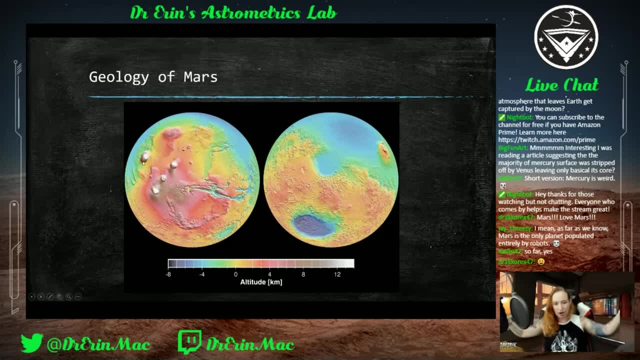 These are all big, huge but broad shield type volcanoes, And then here we have Mariner Valley or Valles Marineris, So those are sort of the bigger features of Mars. Like you're must know If we were doing an exam, 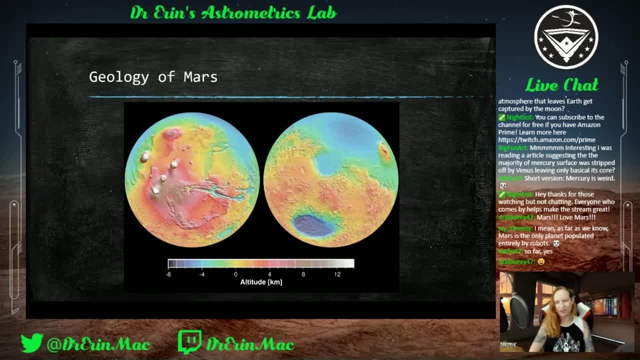 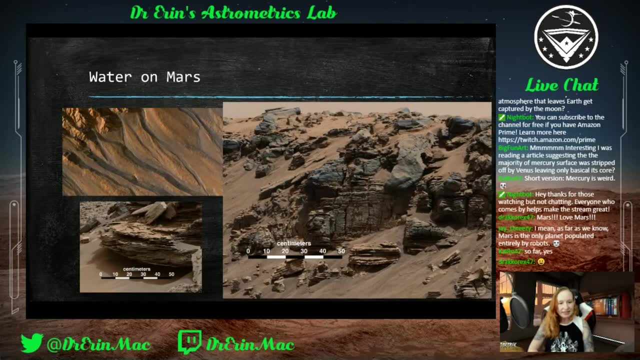 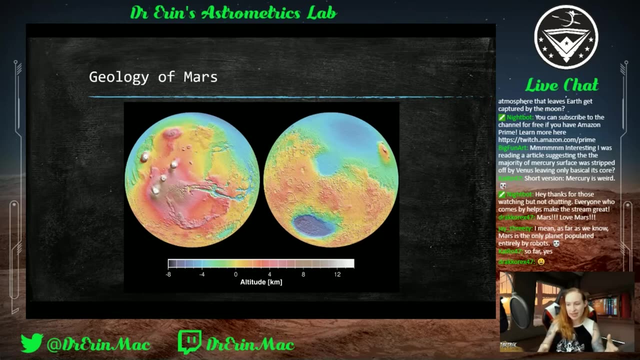 that would be list three major features of Mars: The Tharsis Bulge, Hellas Planitia, and then one of the others. The other ones All right. So that's sort of the general geography of Mars. is interesting It has. obviously it has a lot of history to it. 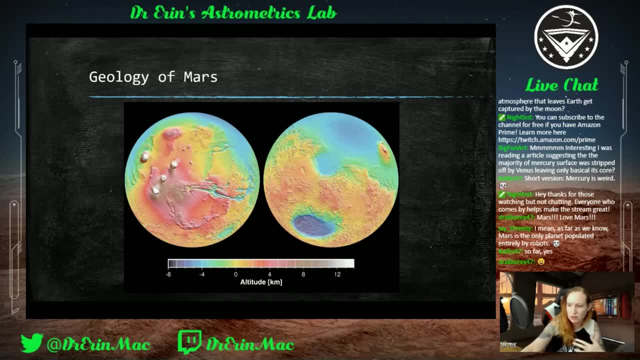 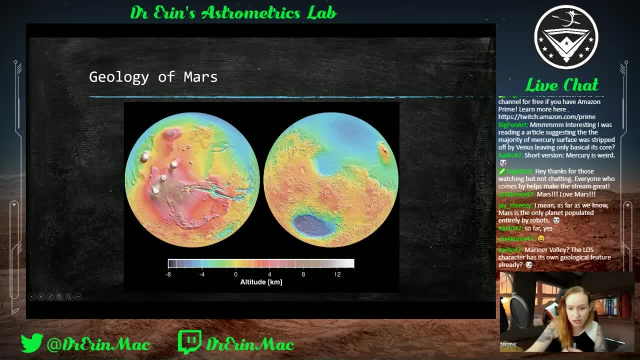 We can see evidence for volcanism. We can see, you know, dead volcanoes here, Massive dead volcanoes. We can also see like a huge crack in the surface that doesn't necessarily look like the Grand Canyon, in the sense it doesn't appear that erosion is what caused it. It doesn't look like the Grand Canyon in the sense it doesn't appear that erosion is what caused it. It doesn't look like the Grand Canyon in the sense it doesn't appear that erosion is what caused it. It doesn't look like the Grand Canyon in the sense it doesn't appear that erosion is what caused it. 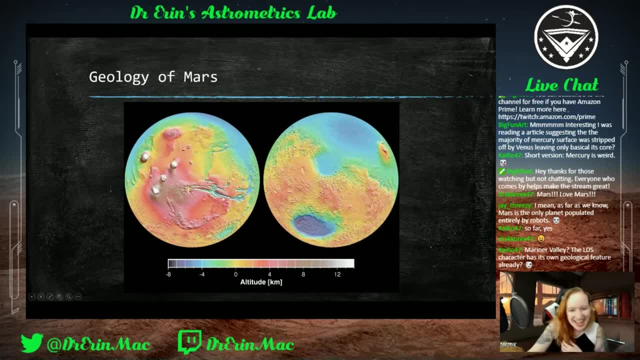 Or maybe it was me that caused Mariner Valley to form. There you go, Kyro. Or maybe Was she named after Mariner Valley. All right, so Vallis Marineris, That's this big crack here. That's this big crack here. 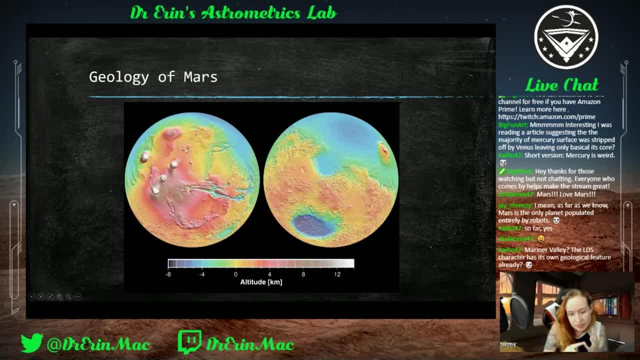 And but there is evidence of volcanism, There's tectonic activity, regardless of what caused this, There's indications of tectonics. And then we obviously especially on this side, And then we obviously especially on this side. 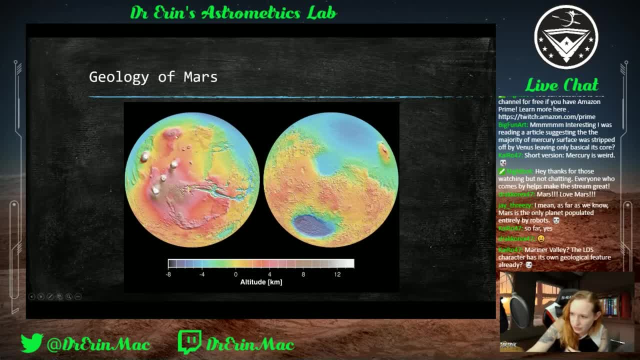 And then we obviously, especially on this side, we have a long time to look at the top. We have a long time to look at the top- a lot of impact craters. The cool thing here is also, you can see how much flatter this. 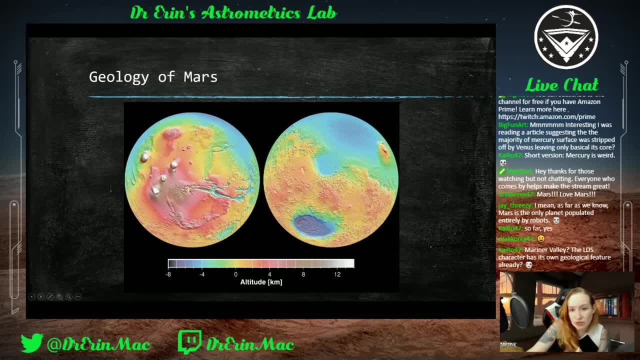 side is That's more formed from the fact that there was volcanism that remember, we talked about how that volcanism can shape the surface of a planet by basically covering up the layers, So stuff, you know, you get these impact craters, but then a volcano goes. 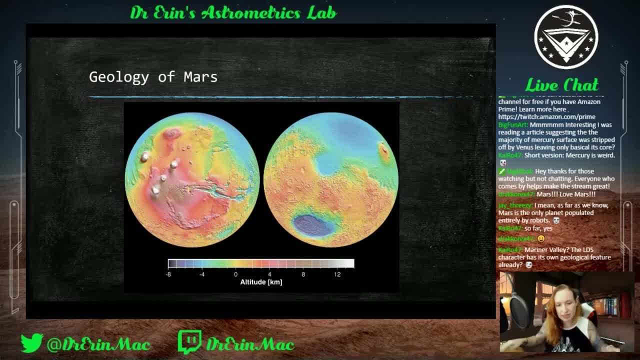 off, and especially the shield volcanoes. all that magma is going to smooth out the surfaces, and so that's kind of what we're seeing here, And that indicates that these volcanoes were relatively young compared to the overall age of, or they at least remained volcanic for. 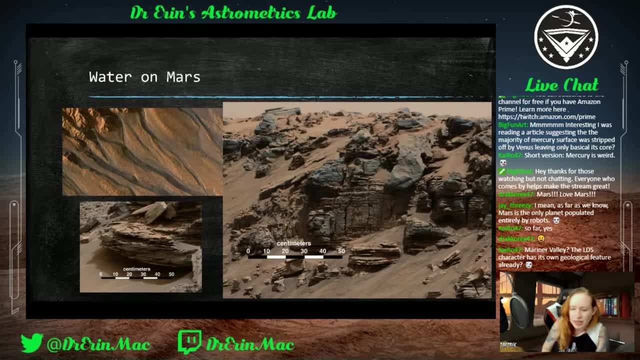 a long period of time, up until recently. Okay, one of the other features that we can see on the surface of Mars is evidence that there was water on the surface. So this is some evidence of water flows on the surface of Mars. This was sort of the first indication. 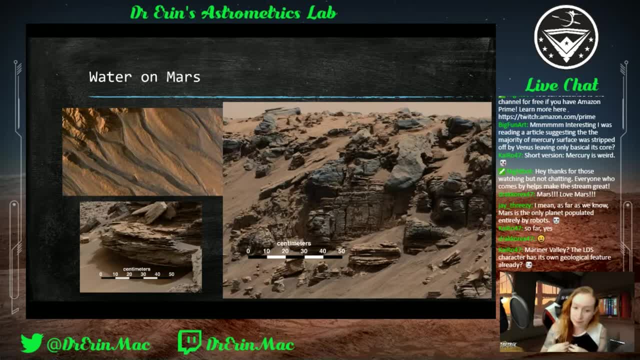 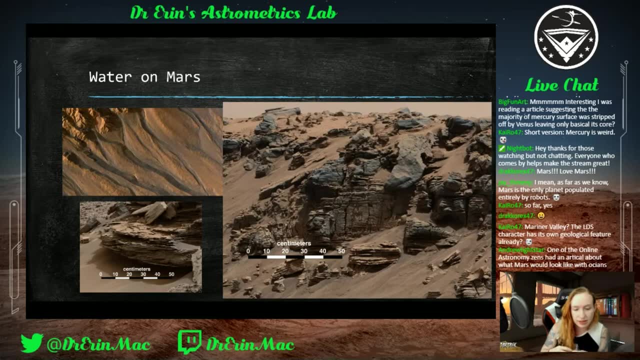 that we had. So when we first started looking at Mars, we thought that it was a lot like Earth, And I just mean through crappy old Galileo-style telescopes- Not crappy, that was mean, But you know what I mean. When we started looking at Mars, what we saw were- and I'll go back- 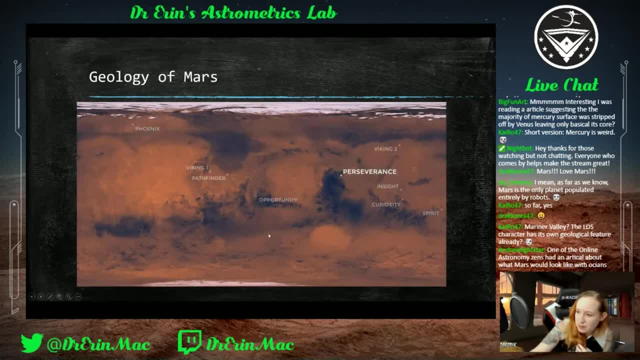 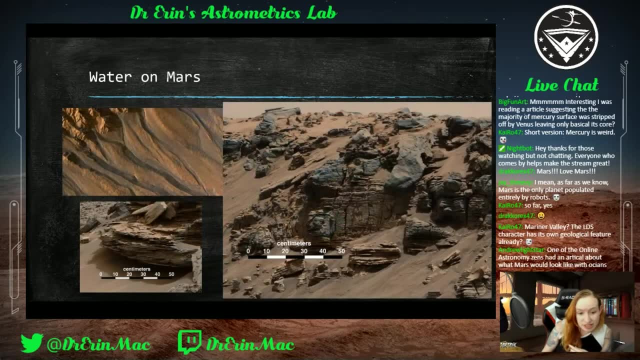 to this. we saw these dark patches, These dark patches here through a telescope- just looked like oceans. So society, society thought that Mars was just like Earth And that's where the idea of Martians came from. They thought that it had continents, oceans, that it looked like Earth because 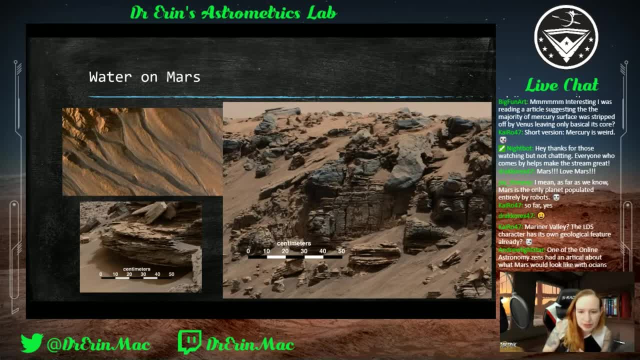 of that And ooh, that's cool, Andrew, I'll check that out. But then we went there and we were and telescopes got better and we visited not humans ourselves, but we sent stuff there, took pictures, realized there is no water on the surface. That made us have. 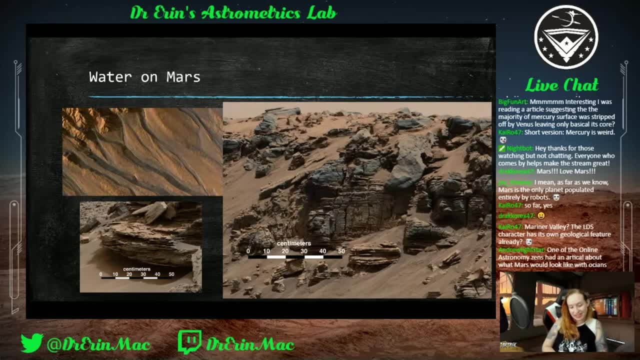 a sadness, But we have found evidence that there was water on the surface at one point first indicated by these, by this- And oh my god, I forgot the word again. I should have put it on here. I got cocky, I said I wasn't OK. first of all we had the water flows, Then actually, 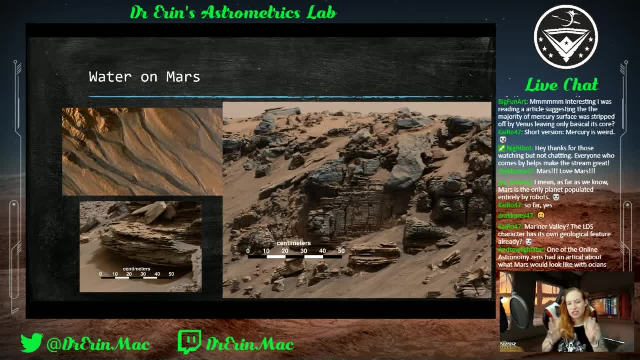 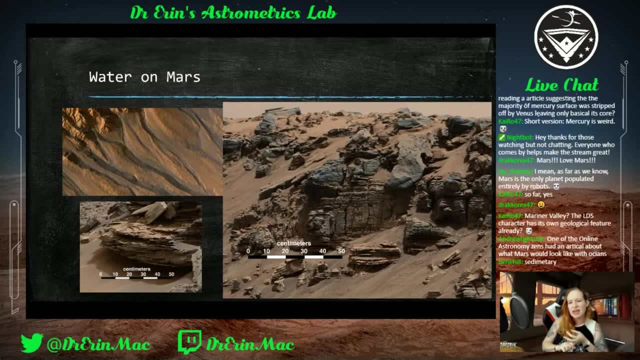 Opportunity, discovered something called- it's a geological term, but blueberries, essentially river rocks- I think is a is kind of a good comparison for that. that. these, uh, thank you, Benny, thank you, you remembered, you knew what had happened, you saw the, you saw the connection fry. 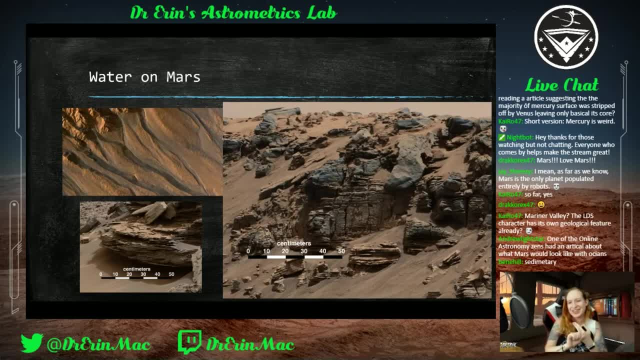 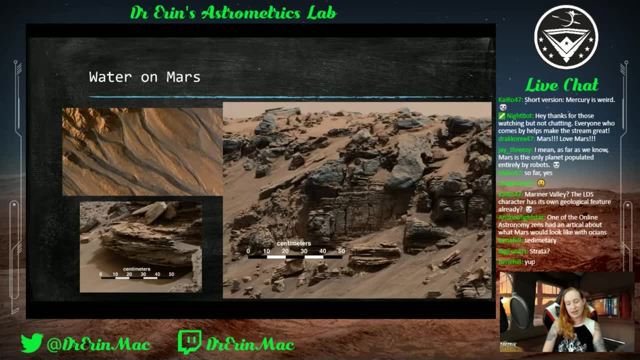 um, uh. so these river rocks, these blueberries that Opportunity saw, were again an indication that there was water on the surface and that there was water flow on the surface. and then, thanks to Benny reminding me, but Curiosity- found sedimentary rock, and that's what we're looking at here. so 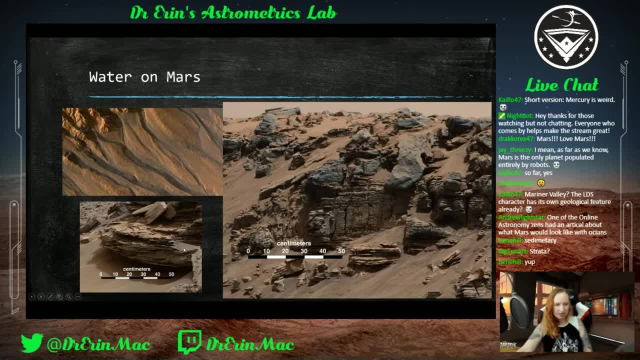 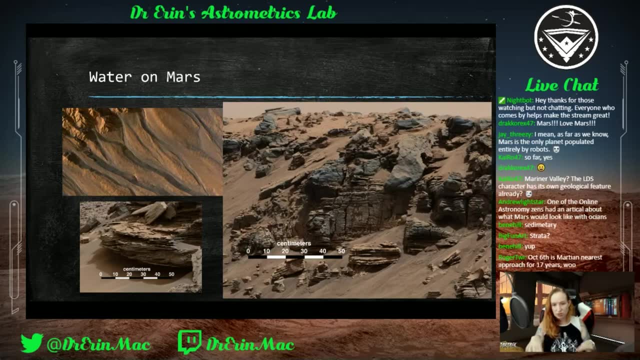 we see the sedimentary lock, these layers, particularly this. I mean this is amazing. this is evidence not just that there was flowing water on the surface, which was everything else, but there was standing water on the surface, that we had these lake beds um. Curiosity is in Gale. 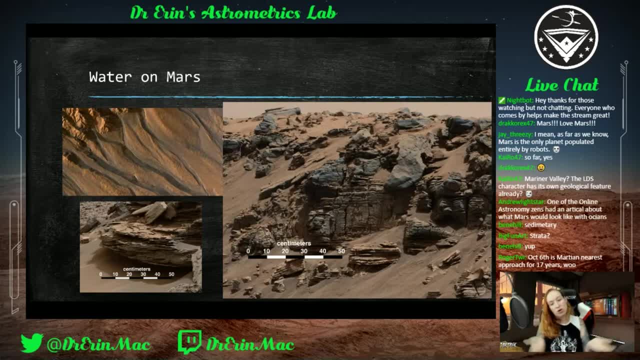 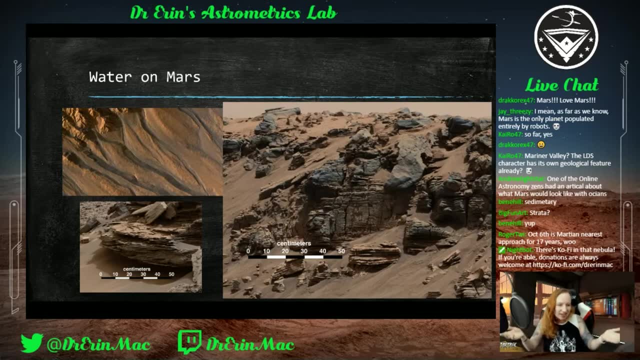 Crater, which is was a good candidate for like, oh, it's a big, deep, shallow area, big deep shallow area, big, wide, not deep and shallow, but it looked like it could. if there was water on the surface it would have pooled in Gale Crater and uh, and so that's why we sent Curiosity there and indeed, 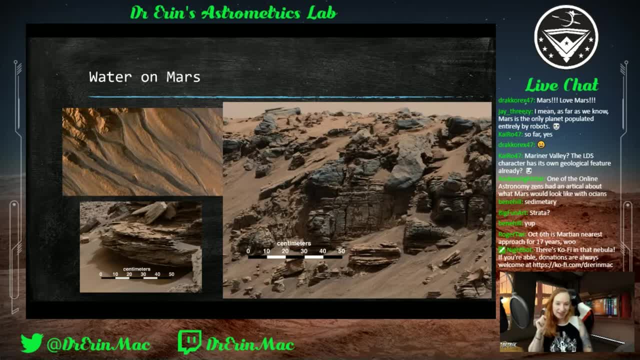 we found this um sedimentary rock- and, yes, I did have to check the chat again so I can remember what it was. uh, and what that is is it basically shows: okay, you have water there, it deposits layers of rock and then that water, you know, there's more erosion, there's more wind blows, the dust in all. 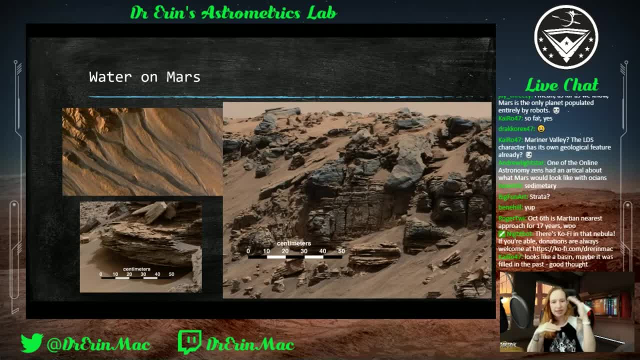 that, and then you have water there. it deposits layers of rock and then that water- you know there's that rock settles again and you just have this repeated settling of layers and you, um, and you get sedimentary rock from that. so yeah, I mean, that was, that was a lot of that reasoning, and then, indeed, 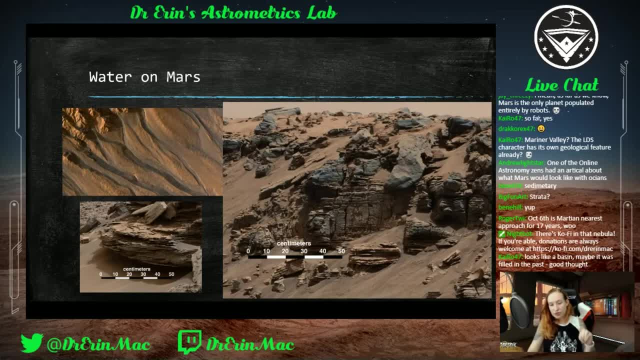 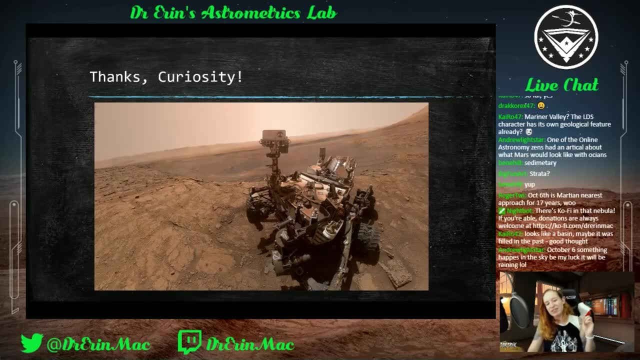 that's exactly what we saw. so we know that there was water on the surface of Mars and we know that there was water for a long period of time on Mars. so thank you, Curiosity. if you ever need a boost, Google Curiosity selfies. you are not disappointed, and um, all right. so what's the? the, the, the, the. 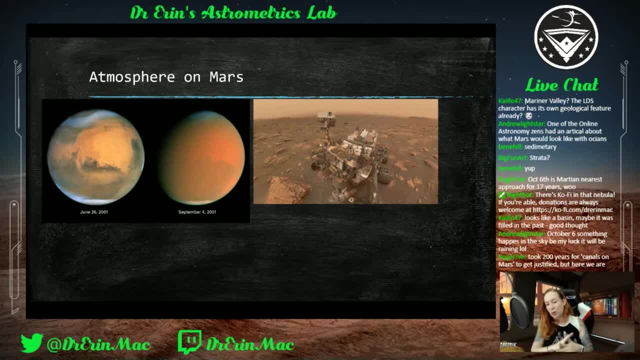 what's the weather atmosphere like on Mars, and then we're going to talk a little bit about what happened to the water, because that's an important component of the atmosphere as well. you may have heard of dust storms on Mars. they can be bad. they can last for a very long period of time, so uh, yeah. 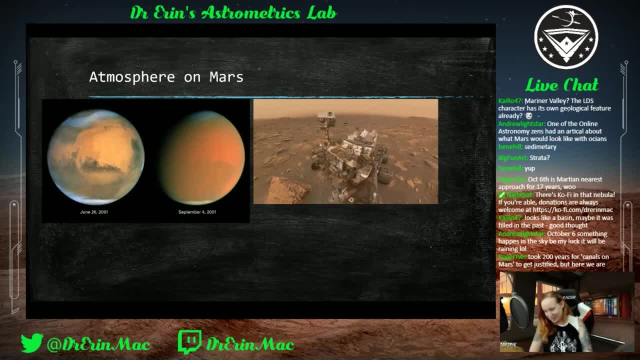 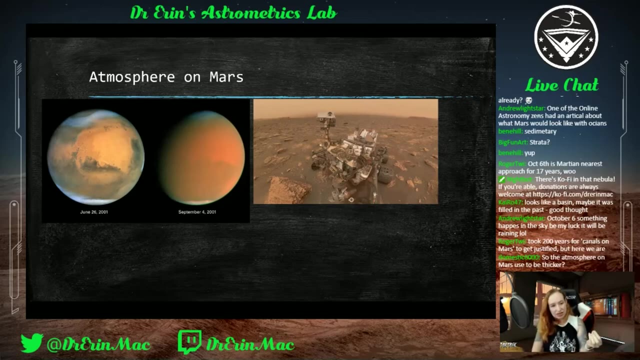 you're not wrong, Roger, that's a. that's a good point as well. the issue is is with the um surface of Mars. it's very rusty. that was sort of that chemical process I talked about earlier. um, that's an oxidation and that dust can can be the um, the consistency of like baby powder, and the gravity. 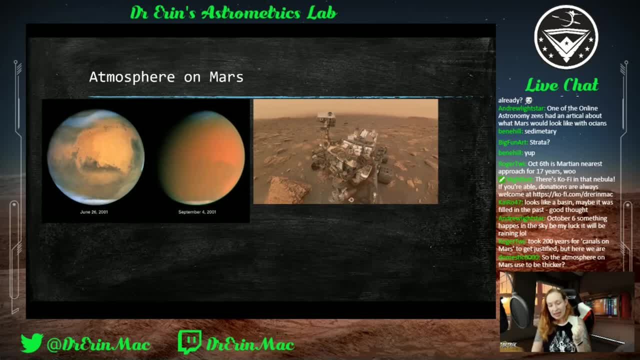 on Mars is only a third of what it is on Earth, and the atmosphere right now is only 0.6 percent, so 0.006 times what Earth's atmosphere is. yes, and domestic- I'll- I'll get to that in a second, but how it is right now, it's only 0.6 percent. it's very, very, very thin. 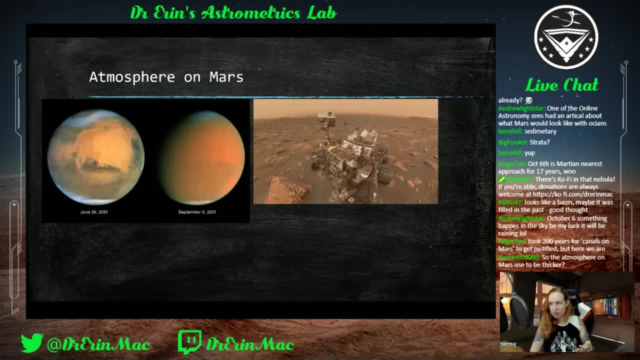 but it's not non-existent. it is there and we do get dust storms. this is another Curiosity selfie, but you can actually see the dust storm behind it. this is the dust storm that covered up opportunity solar panels, resulting in the loss of contact from opportunity. and uh yeah, so these dust storms do. 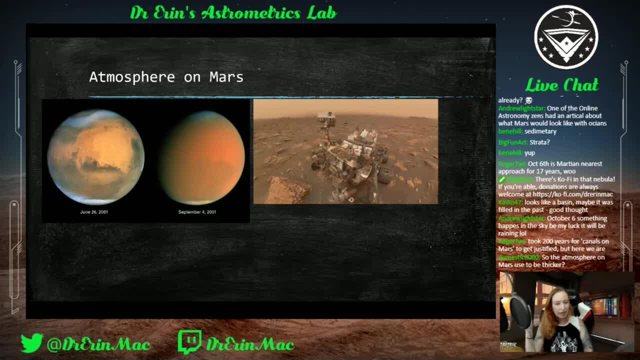 happen, but it's important to note and if you watched my episode club about the ocean, because the atmosphere is so thin, when these dust storms happen they kick dust up, but that dust doesn't actually that you don't feel the wind, because we feel wind from the pressure. 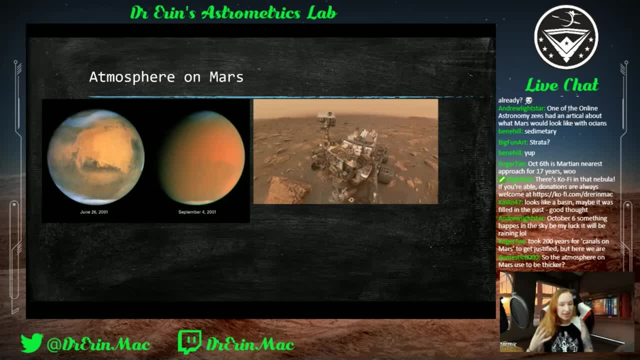 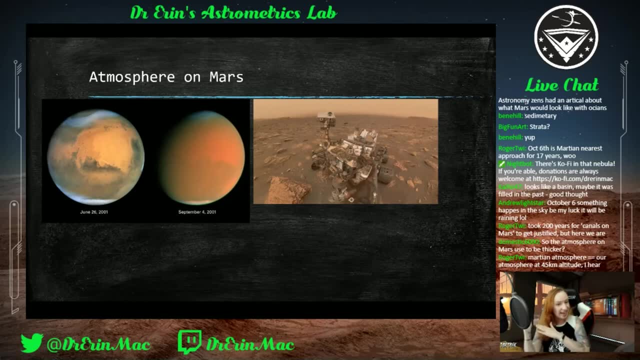 of atmosphere pushing on us. Mars doesn't have a thick enough, enough atmosphere to actually push us or knock over you know a rocket, or blow a satellite into Mark Watney. it just it kicks up this really, really thin dust and then it takes a long time for it to be settled. 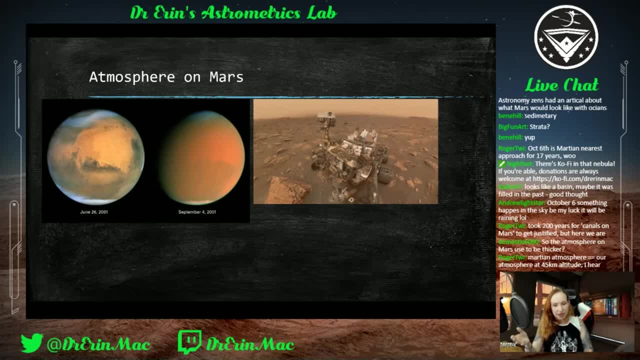 down and uh. yeah, Roger, that's a great comparison. our atmosphere at 45 kilometers, which is really really high, is, uh, is about equivalent, so that's a that's a great point. um, and then there is some cycles of weather on Mars as well. this is an animation of the North Pole on the left, and 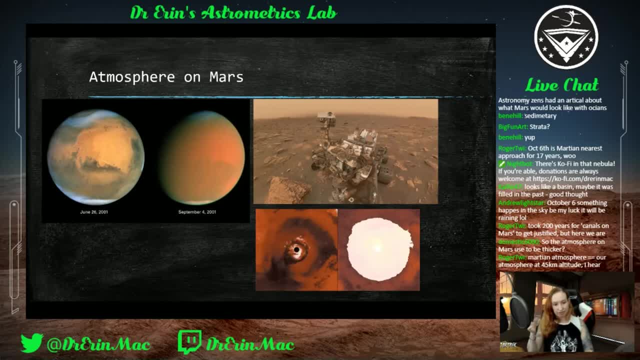 the South Pole on the right over the course of a year. so there is a sublimation and condensation. that happens. remember, this isn't raining. this isn't melting into liquid. this is a solid evaporating into a gas. this is dry ice, this is carbon dioxide primarily, and it evaporates. 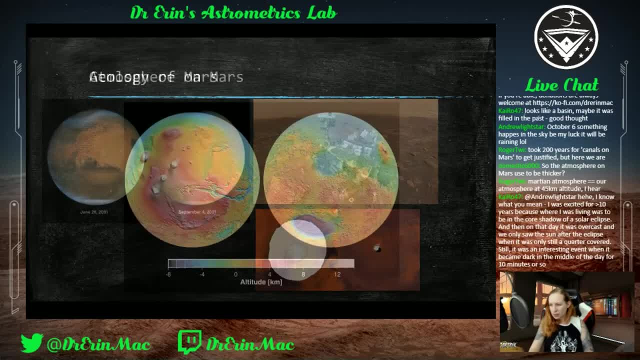 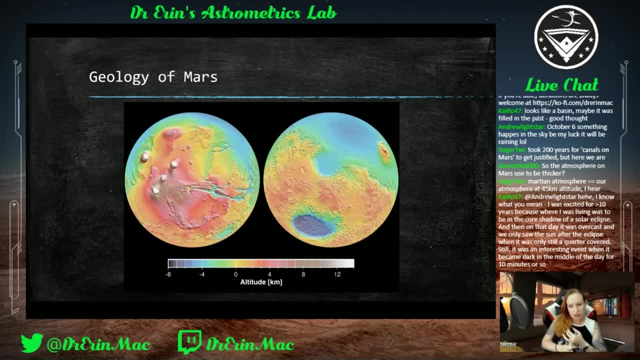 and then it condenses and goes back down. okay, so what happened to Mars? and domestic kind of hinted toward this a little bit. we know that there was standing water on the surface of Mars. because of that, there has to be an atmosphere. atmospheric pressure is what allows water to. 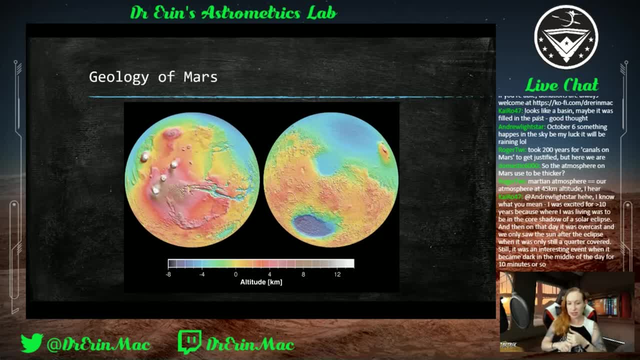 remain in liquid form. if you've done this experiment at the science museum, where you can put a little cup into a vacuum jar, suck all the air out, the water will start to boil, not because it's hot, because there's no atmosphere holding it down and keeping it in liquid form. so in order to have liquid water on the surface, you need to. 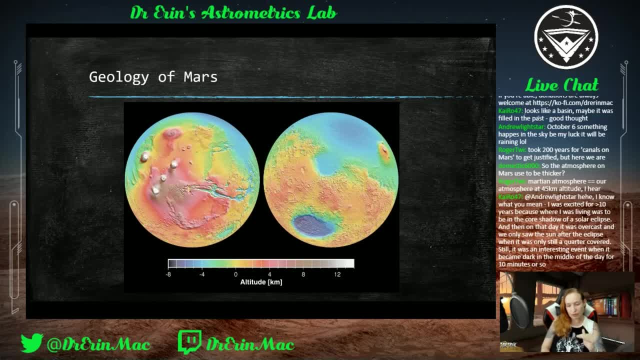 have an atmosphere that is thick enough that it keeps it in liquid form, and that had to have been the case for Mars. now, what the atmosphere is right now would not work. if we took a cup of water out onto the surface of Mars, it would boil away, it would evaporate. so that means if there was liquid, 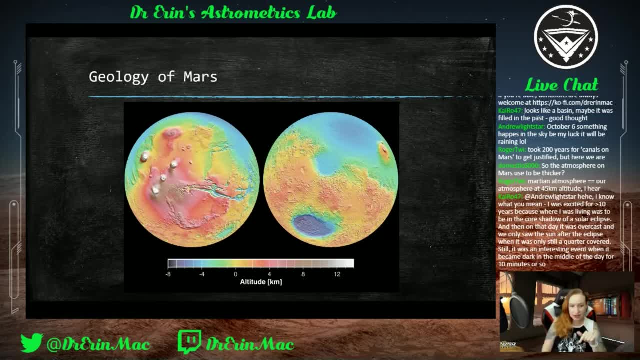 water on the surface of Mars. in the past it had to have had a thicker atmosphere, and this is something that the messenger spacecraft is going to study, that that is studying right now, that it is studying, um, what happened to Mars's atmosphere. it's trying to study the proportion. 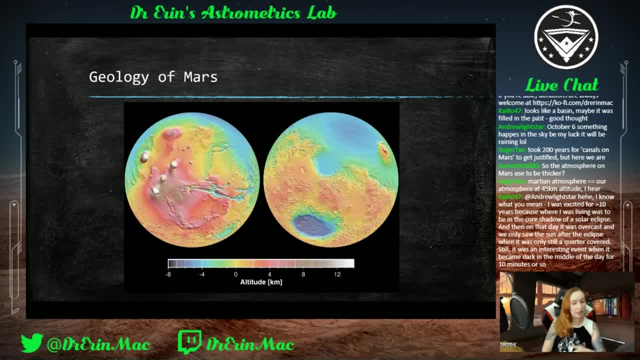 of the atmosphere, really get a lot more detailed readings on the molecular distribution to see if the atmosphere slowly disappeared over a period of time or if it was like a quick impact that caused a lot of it to disappear. and when I say impact, that's what we're talking about here. 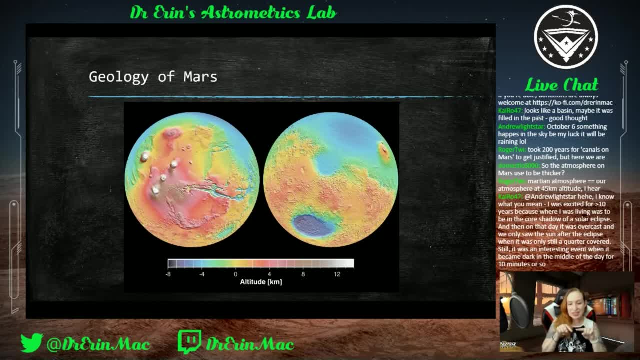 now remember: in order to keep an atmosphere, you need to have a magnetic Field. this is all tied together and that's what we talked about last week: how a planet can have a magnetic field. it needs a molten metallic core. that molten metallic core, as it rotates, gives off a magnetic 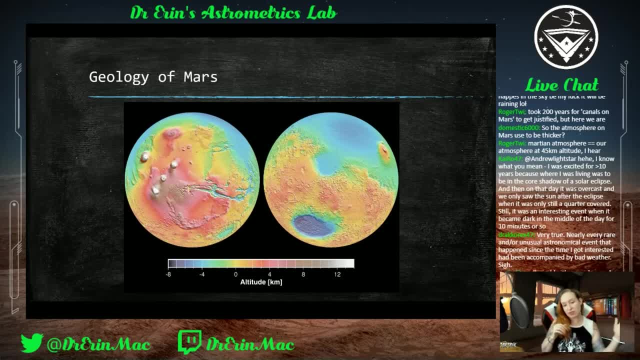 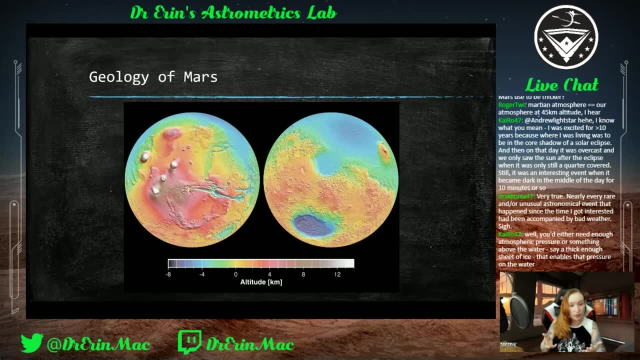 field that magnetic shelters the atmosphere from solar winds blowing it away And that atmosphere will keep liquid water liquid on the surface. So it's this whole cathodate, the rat chain. You need a magnetic field to protect the atmosphere, to protect the liquid water. Um so, uh yeah, And Cairo said you'd. 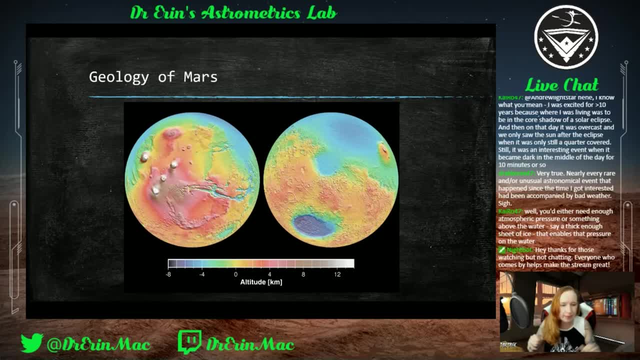 either need enough atmospheric pressure or something above the water like ice. Yeah, I absolutely, And uh. but the question is so: what happened? what happened to that magnetic, the magnetic field? What happened to the core of Mars that caused that to happen? 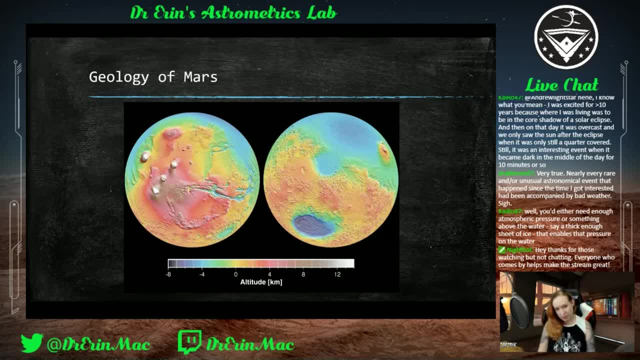 There's two theories, Um one's more apocalyptic than the other. That one I like the most, but the the one that's, I guess, because there's no evidence, there's no direct evidence. We haven't, we didn't see it happen. Um one of them is okay: Mars is half the size of earth. 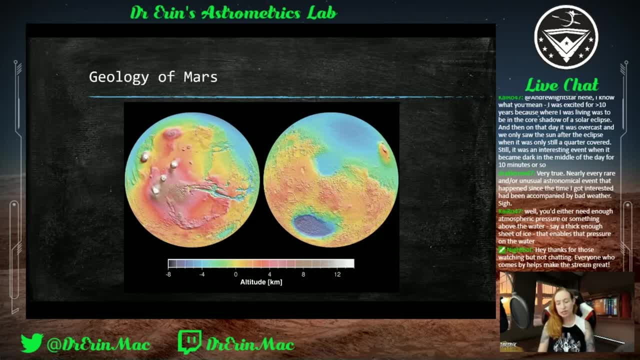 just cooled off. It's just like mercury, You know, mercury cooled off, Mars cooled off. uh, the interior just solidified and it lost its magnetic field. because it's half the size, You take two loaves of bread out of the oven. 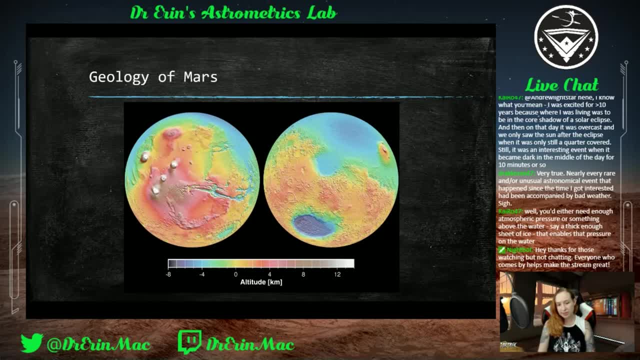 one half the size and the other the one that's half the size, is going to cool off faster. Once it cooled off, that magnetic molten core solidified, no more magnetic field. atmosphere goes away. water evaporates. I like my theory better. It's not just mine, but um. 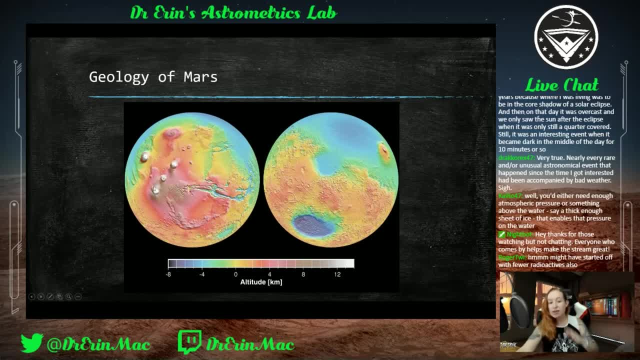 this is Hellas Planitia. This is the Tharsis Bulge. Hellas Planitia is an impact crater. This is a massive impact crater. It's the largest visible crater in our solar system that we've seen. It's crater has craters and those craters have craters. 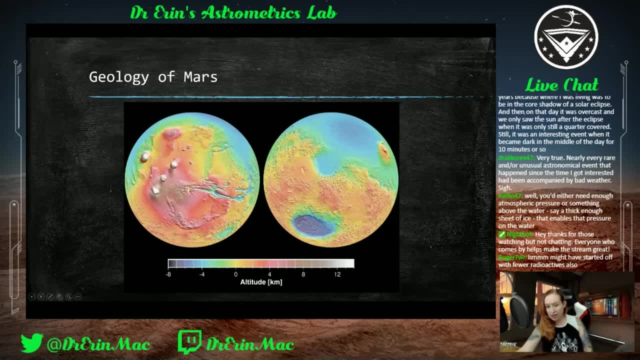 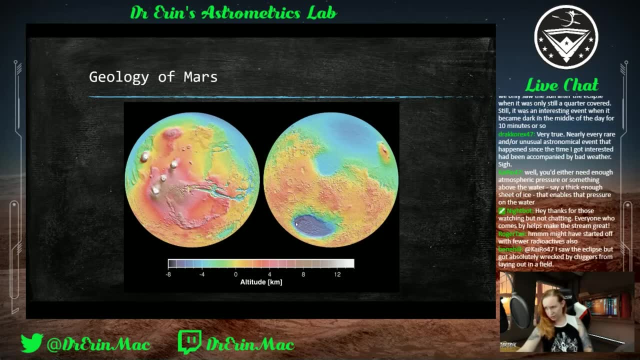 So this crater here is directly, almost directly opposite from the Tharsis Bulge. Um, so the Tharsis Bulge, we think, is caused by an impact crater hitting here and bulging out the other side like brutally causing a crack, causing massive. 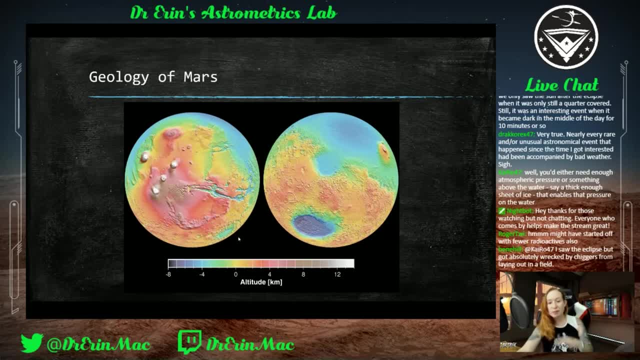 volcanic activity that then also completely disrupted the magnetic field, completely disrupted it Um. that disruption caused it to just become unstable and solidify off a lot faster. Solidified magnetic field disappeared, atmosphere went away, water evaporated. So those are the two kind of big, big theories from Mars, And it's awesome. 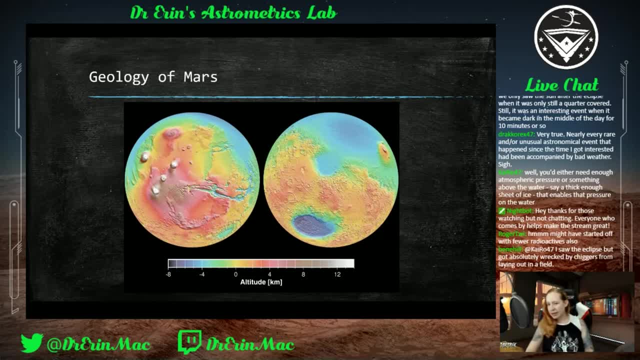 and cool and exciting. Okay, Now then. yeah, Roger, actually that's a really good point too, that um might also have started out with fewer radioactives, And, uh, yeah, everyone's sharing their sad astronomy experiences that were ruined by weather and clouds. 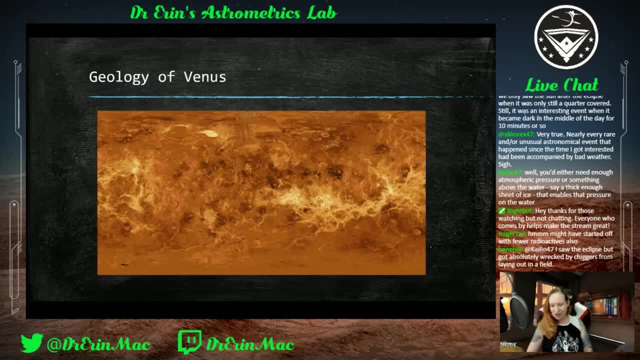 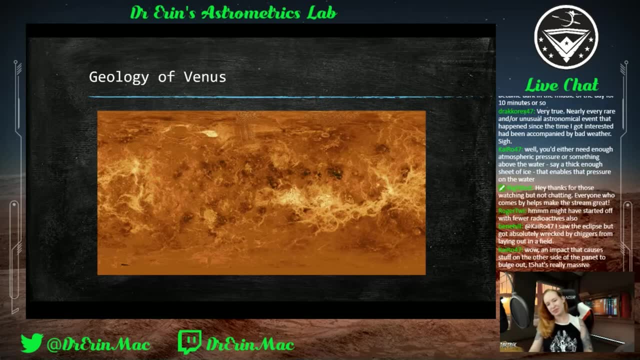 It happens. All right, now we're just going to wrap up. We're pretty much going to go the whole hour, so I apologize for that. We're going to wrap up. We're going to wrap up with Venus. Um, now I could- uh, I could- talk about Mars for a lot longer, because it's really really cool, but I wanted to end with Venus just because I have something really geeky and adorable and amazing to talk about with Venus. 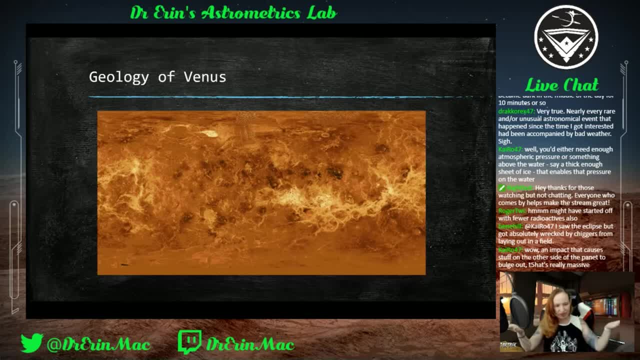 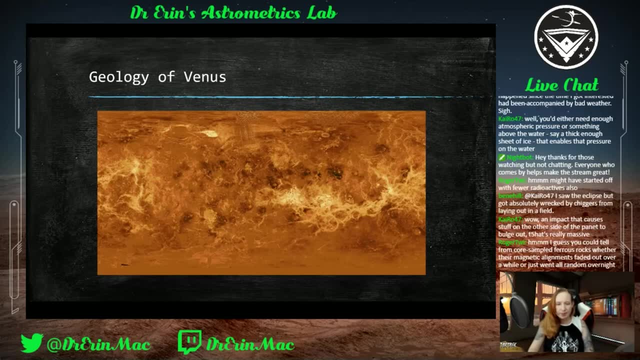 But, uh, this is again kind of blown out, uh, picture, flattened out picture of the surface of Venus, mostly taken through radar images. Taken through radar images, Not mostly. Um, yeah, Roger, that's, and that's exactly something that I'm going to be talking about. 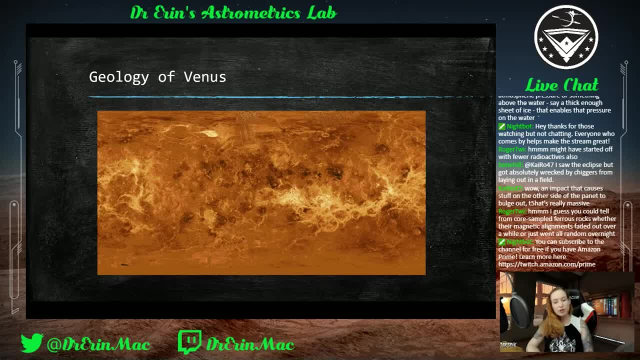 Um, so, um, I'm going to wrap up with Venus. That's exactly something else that they're going to study. That's, I think, what Curiosity has been taking core samples. Um, remember, Curiosity has like that mole thing. 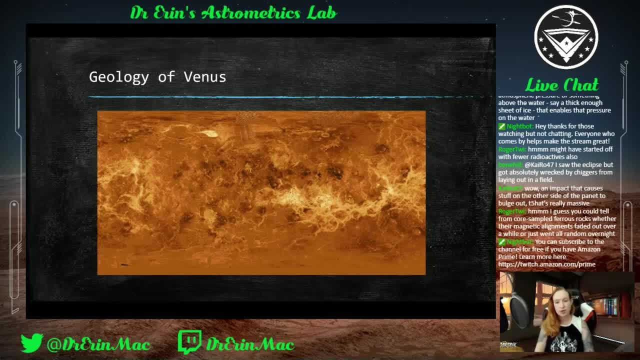 And then I think Perseverance has the same type of instruments. So taking these core samples, trying to study what the interior looks like, will give us clues to that history as well. It's just an unknown. We really, we really don't know. 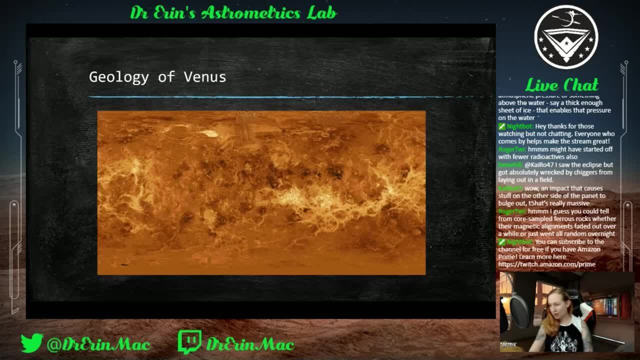 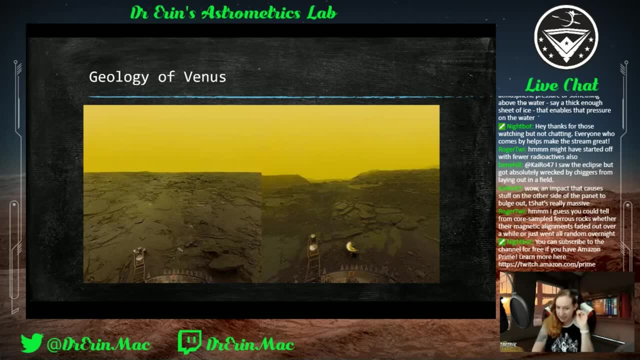 So, um, that's something that we're still studying. All right with Venus, um, looking at the surface of Venus, this is: these are the Venera landers That um made it actually made it through the atmosphere. 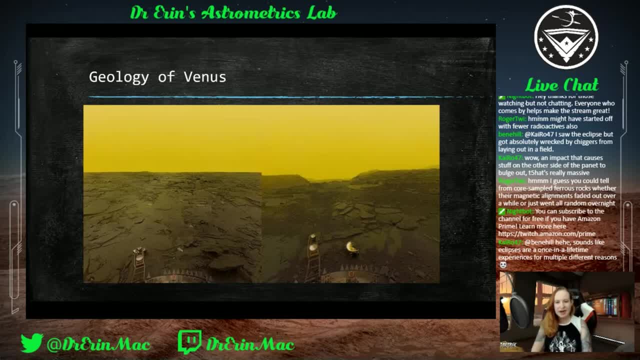 The atmosphere of Venus is a unique beast, So um it. these are pictures of the surface of Venus- High volcanic activity. I feel like there was something else I was going to say about Venus that I don't remember off the top of my head. 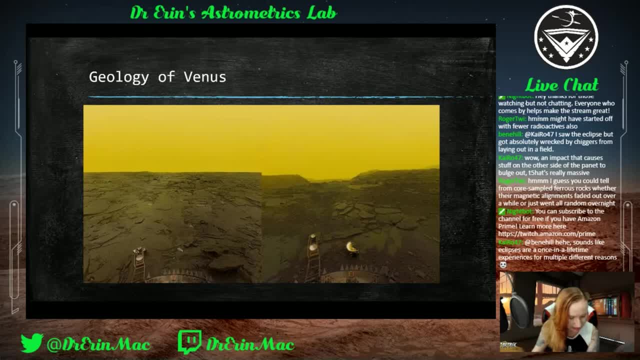 Um huge amount of volcanic activity, Large amounts of outgassing- Our favorite word, And um, yeah, I think that was. that was amazing Major thing. Let me see if there was anything else. It's really the atmosphere. that's the important part with Venus. 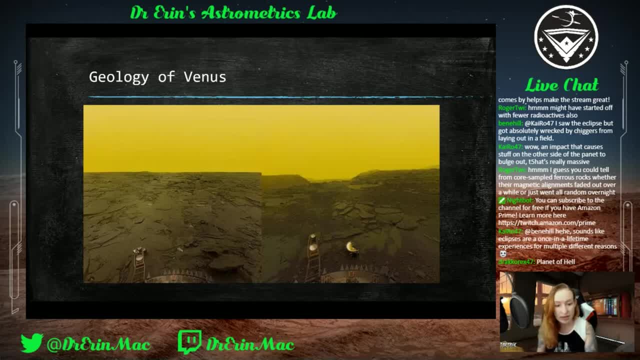 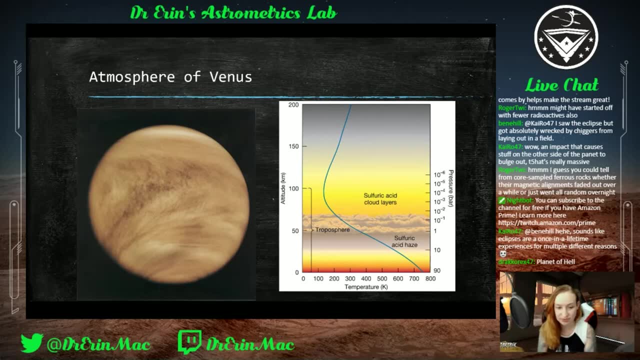 Uh, yeah, The hell planet Agreed. Uh, the atmosphere is really what screws us up, Because Venus is about the size of of Earth. It's um, it's almost 1G, I think it's like .9G times the gravity. 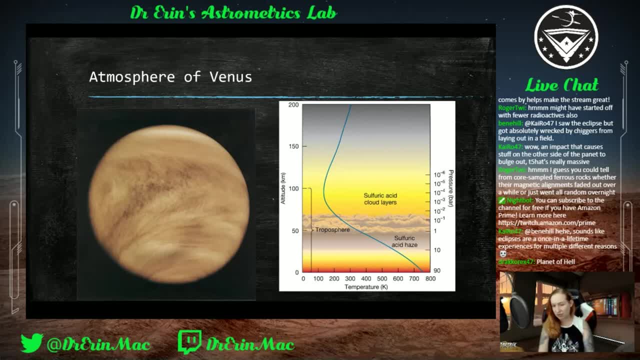 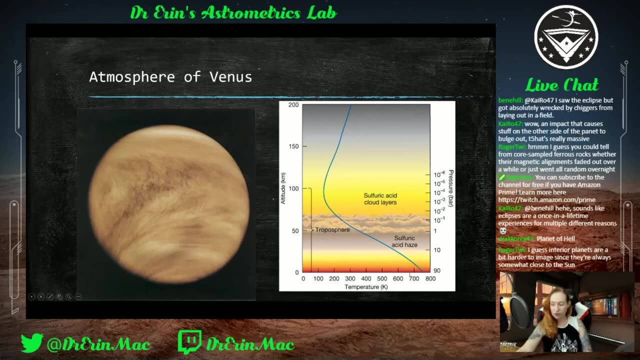 Uh, so like we could walk around on the surface of Venus pretty well, Except for the darn atmosphere Breaking out these, these layers again. Um, you can see right here, This is 90 times the surface of Earth. So this is the atmospheric pressure. 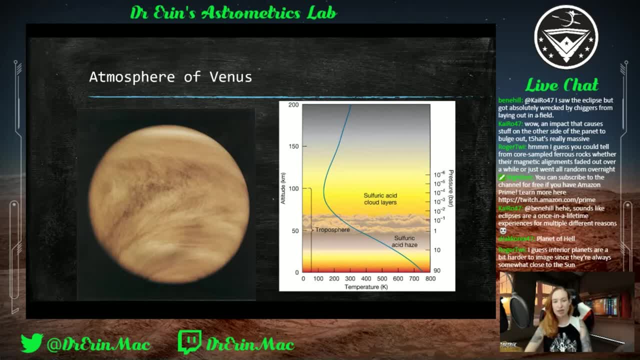 90 times, Nine zero times. If you took the column of air above me, Added all that up into a weight About the weight of a car. Now turn that into 90 times. That just squishes you. Um, yeah, and Roger, a lot of the imaging actually is mostly um, because of the clouds. 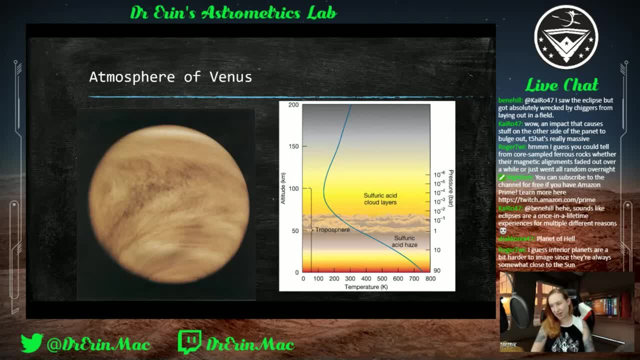 That's why we needed the radar. It's got really, really thick clouds And it's sulfur, Mostly sulfur. Not pleasant, Not good for us. Sulfuric acid in the atmosphere, High amounts of sulfuric acid, Huge amounts of carbon dioxide. 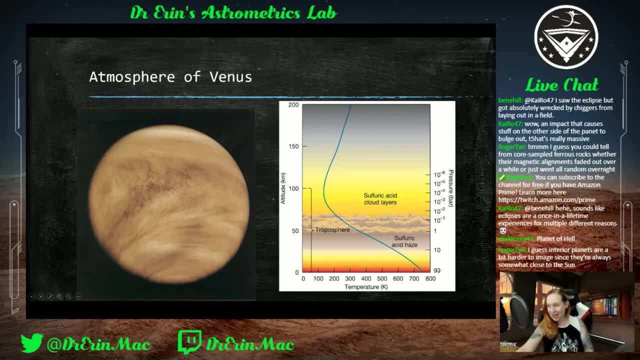 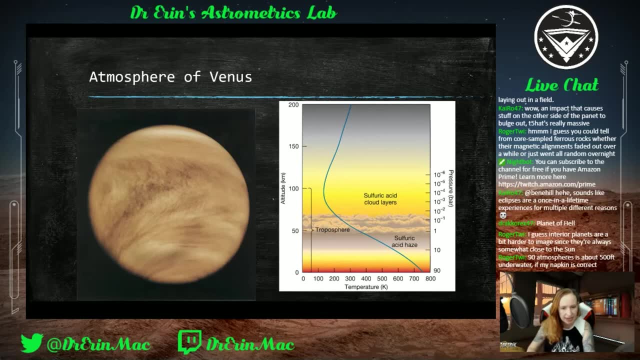 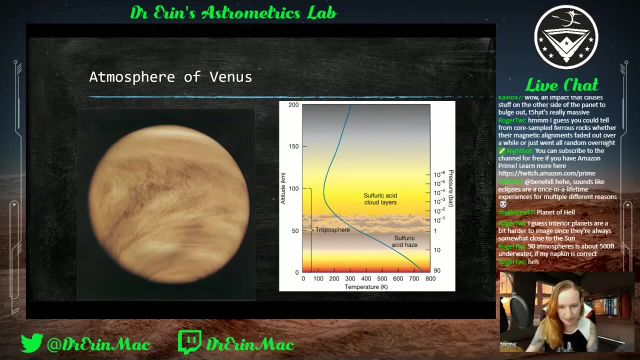 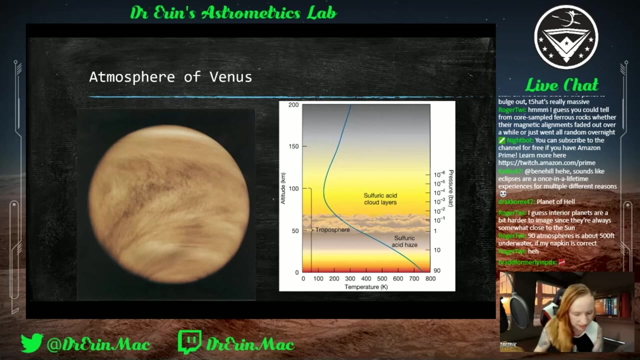 Very, very, very high temperature, High density, High atmospheric pressure, Because this pressure is so high. The temperature, um, yeah, it's actually. thank you for that. um, I did have that number. I have that number. just give me one second um for how deep you would have to swim to get 90 times the um pressure. I think it's about a kilometer under the surface. so, yeah, um, yeah, it's not ideal and uh, yeah, you'd have to go about, uh, one kilometer under the surface of water. 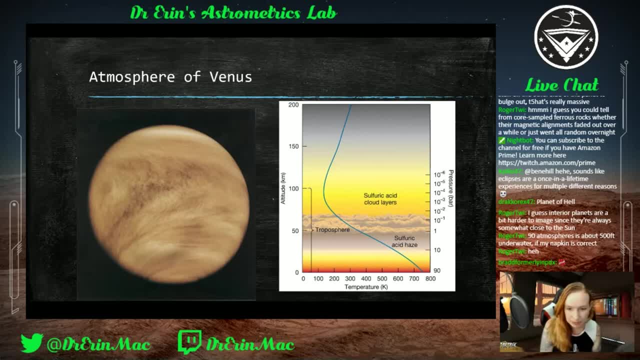 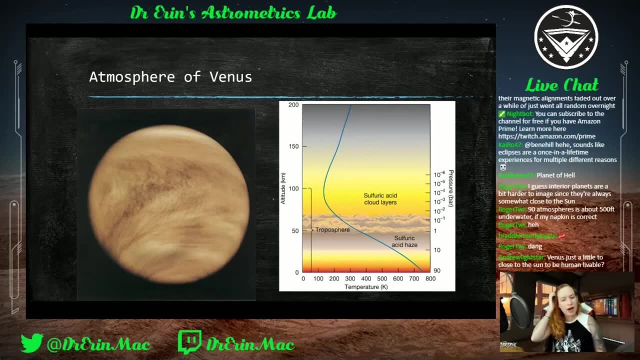 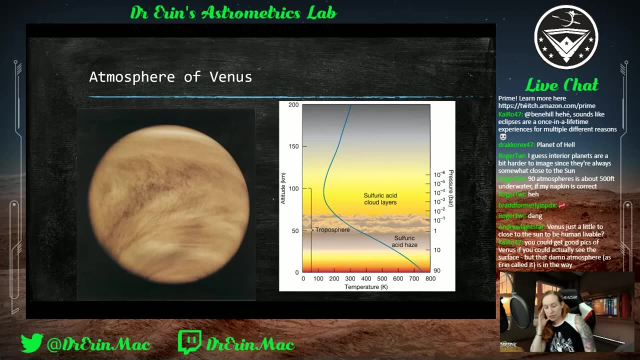 To get that same atmospheric pressure. Not pleasant, Not ideal. And uh yeah, 0.6 miles. So yeah, Um, the temperature, so it's more. the temperature is just too high, Not so much because when we talk about the Goldilocks zone and the temperature, I think Venus is technically a little too close to be warm, but it's but it is. its atmosphere is highly reflective. 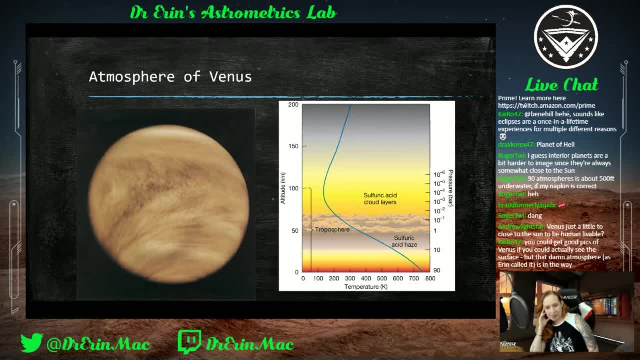 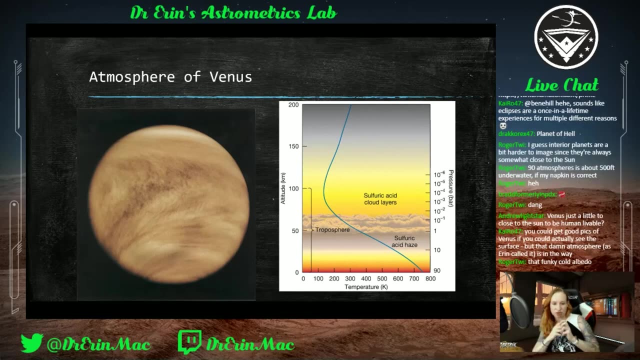 So I think that that cools it off as well. Um yeah, and that damn atmosphere collapsed. the first few landers we tried to actually send to image the surface When we tried to throw something through the clouds, not necessarily knowing how dense it was- they just went and, um, destroyed themselves because it was way too, too stressful. 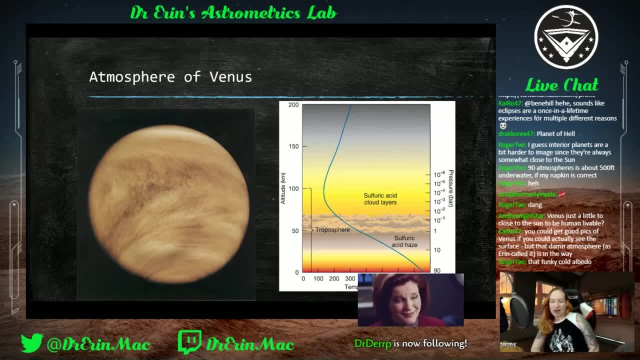 Oh, thank you, Dr Derp, Appreciate it Right. Because the pressure is so high That caused Causes the temperature to go up, Remember? I mean, this is kind of a physics thing: If you increase the pressure, the temperature is going to cause is going to go up. 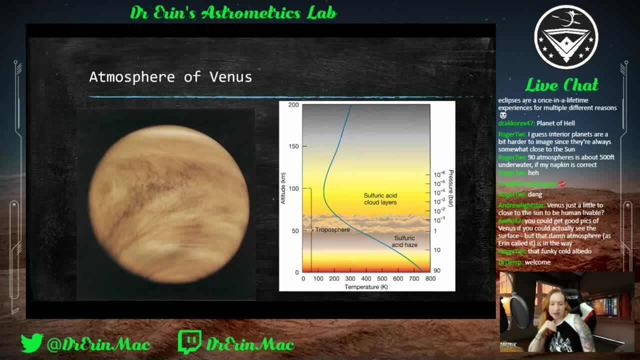 And so the temperature on the surface as well. it's not. I mean, you could keep it in like there's so much uh atmospheric pressure to keep your water in liquid form, but then it's so hot that it's going to evaporate out. 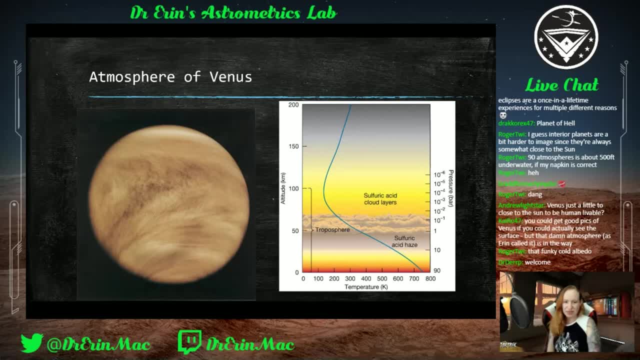 So it's a delicate, delicate balance. But the keen-eyed among you may make note of something: It depends how well you know your, your uh Kelvin temperature. average temperature on earth is about 300 Kelvin ish, um about 288.. 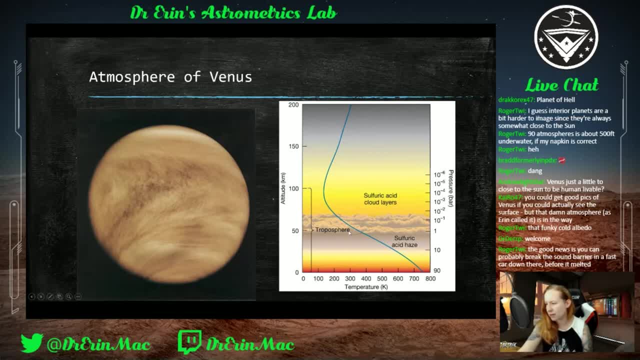 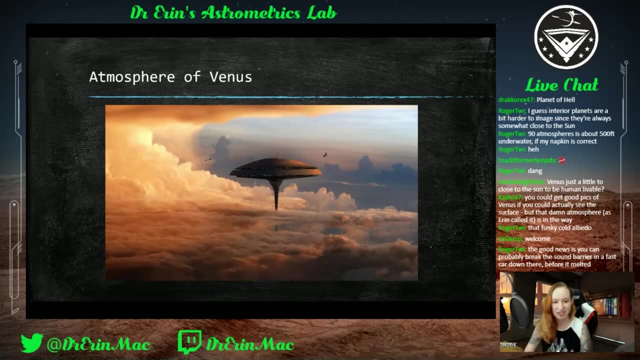 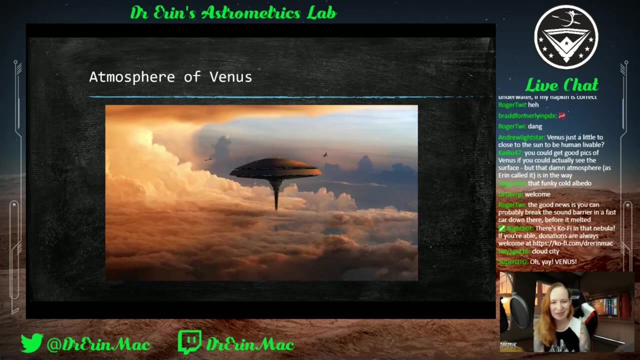 I think, if you follow this up to where, you get one bar of pressure. So this is about where earth is. Does it give anyone ideas? Cause it gives me ideas to build a cloud city in Venus, And this is something that has been floated, floated before. 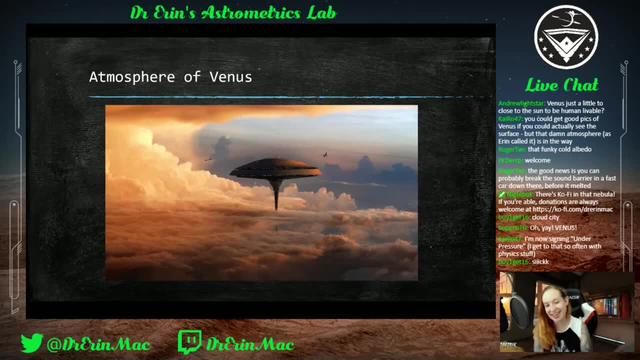 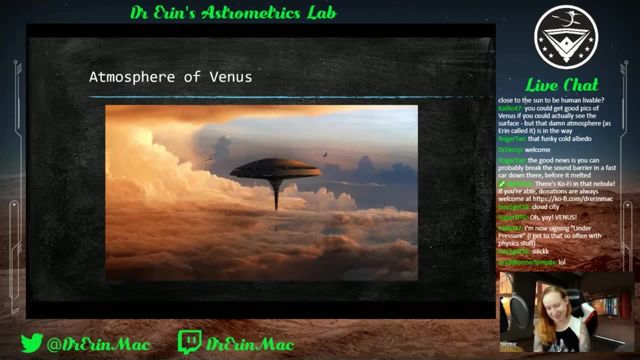 So, um, unfortunately you can't necessarily breathe the atmosphere because that whole sulfuric acid thing is not ideal, but uh, yeah, super cool, Super fun to think about And uh, I love this idea and I hope that we do it because I want a cloud city. 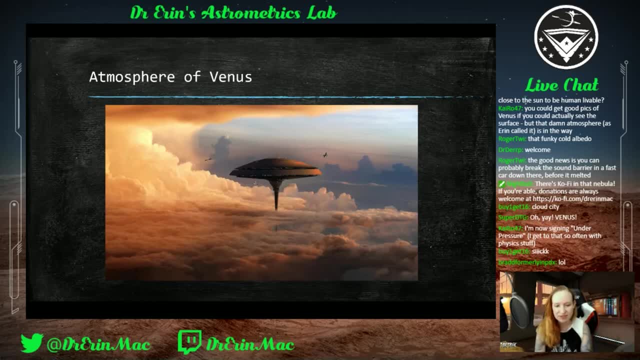 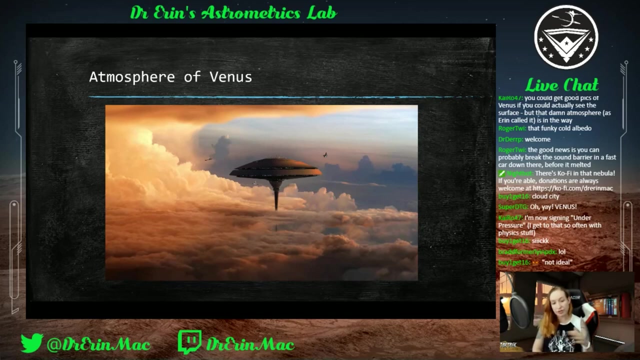 Uh, we talked a little bit about the greenhouse effect before as well. Um, Venus has something we call a runaway greenhouse effect. So earlier we had a question about the equilibrium with atmosphere. The amount going into it is the amount leaving it. Uh, the Venus, when it comes to the temperature, is what we call a runaway greenhouse effect, where we have, especially on the surface, it's continually trapping air. 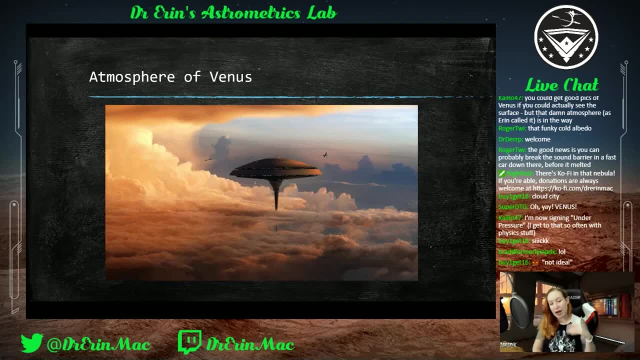 Um, it's continually trapping heat. I talked at the top about how greenhouse gases work, The fact that they absorb infrared radiation, And then It's going to re-emit it, and the more of those that you have won't let that heat leave then, um, it's just gets hotter and hotter, and hotter. 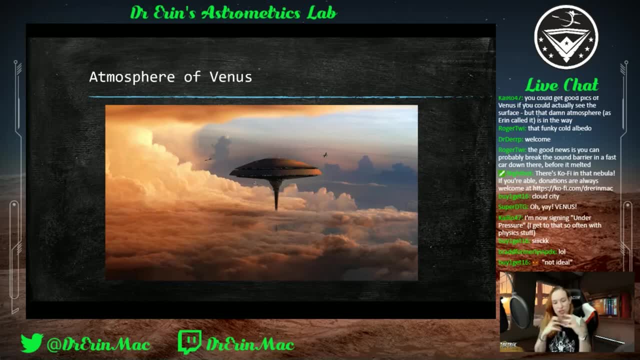 And then, as that heat increases, it's going to evaporate, It's going to split more molecules, It's going to create more greenhouse gases that are going to trap more atmosphere, And so that's this runaway effect And uh, so it's really important to think about. 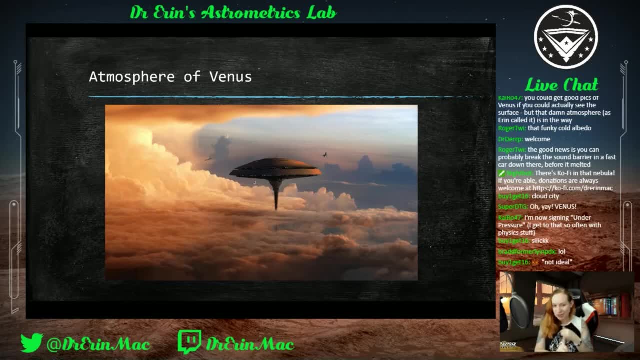 So if you'd like to learn more about this stuff, I can recommend the Futurama episode crimes of the hot high recommend. Also, if you can find it- I don't know if it's on Netflix still- but the new cosmos, the Neil deGrasse Tyson cosmos, has a great episode on Venus, greenhouse gases, climate change, the difference between climate and weather. 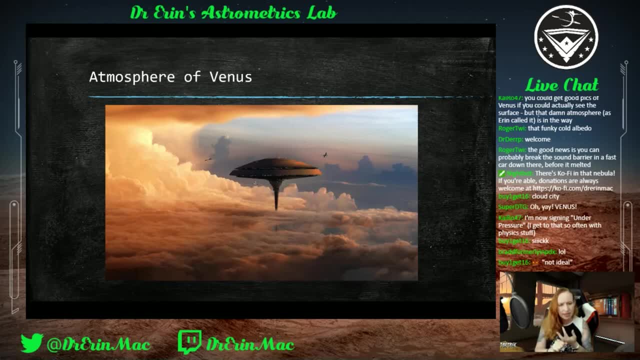 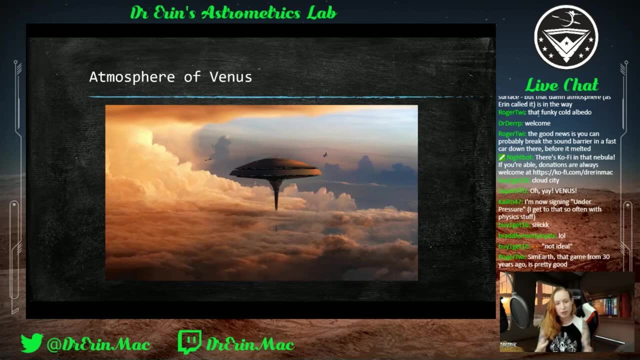 And I would say as well, you know, I kind of I said that we weren't going to take the whole hour to talk about climate change here on earth, because that's a whole other conversation, but it's an important conversation. So, if you aren't sure, if you've been confused, if you're not, you know, if there's a lot of information.